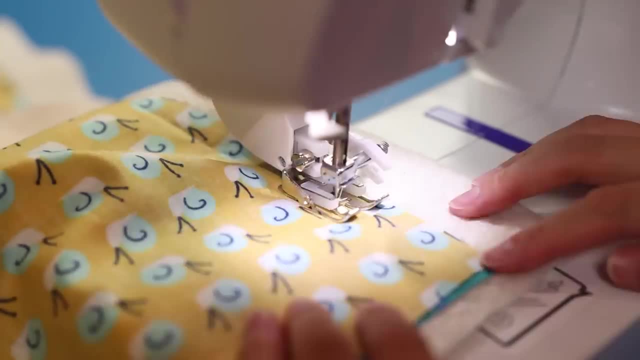 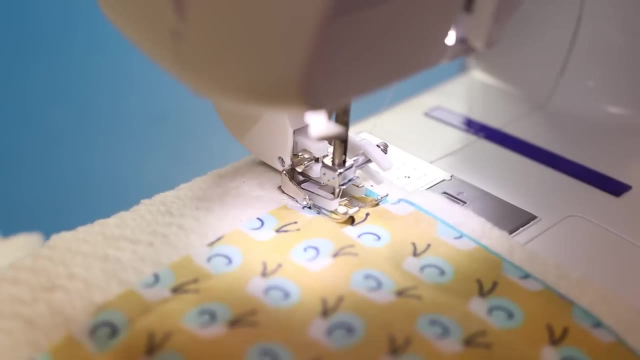 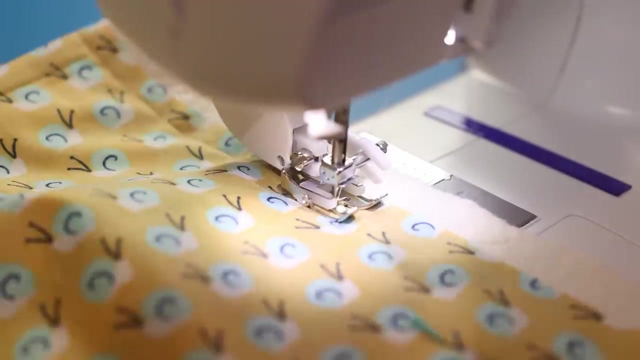 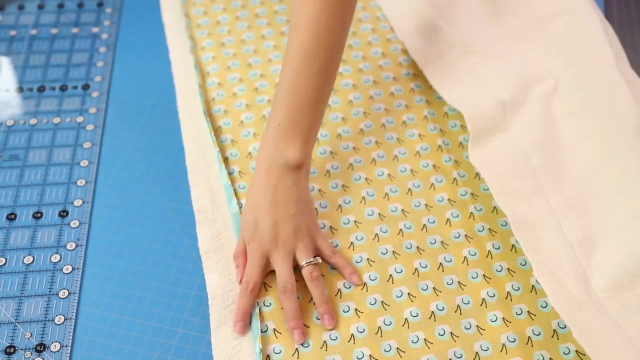 allowance At each corner. leave the needle down and pivot 90 degrees. Continue sewing down the next side. Leave about an 8-inch opening for turning. Here's how I trimmed the excess batting: Fold back the seam allowance, then turn the fabric inside out. I'm going to be using a 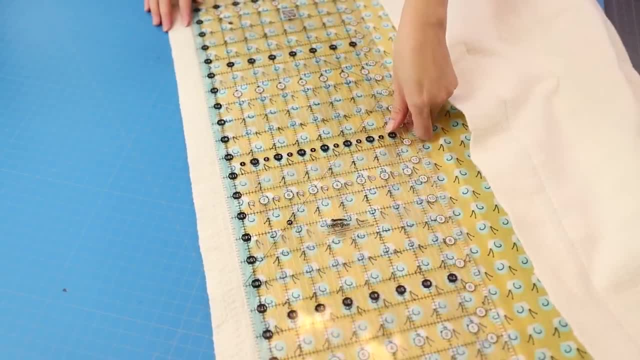 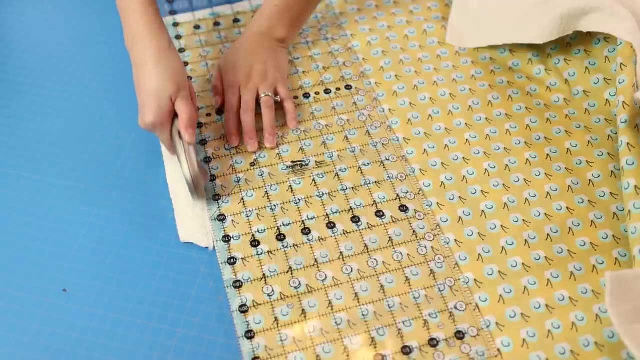 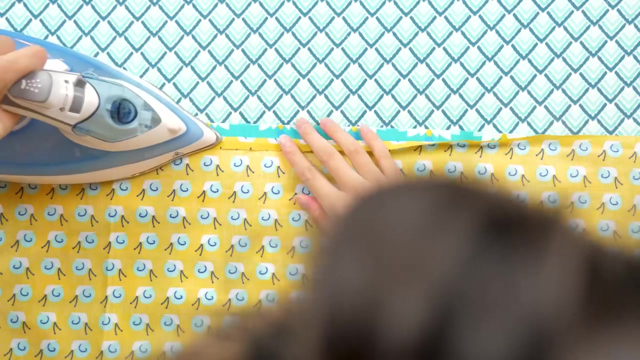 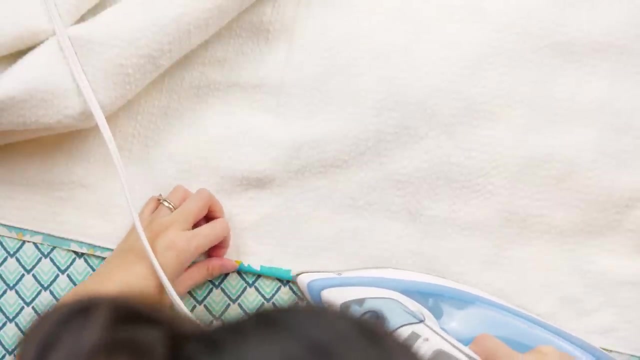 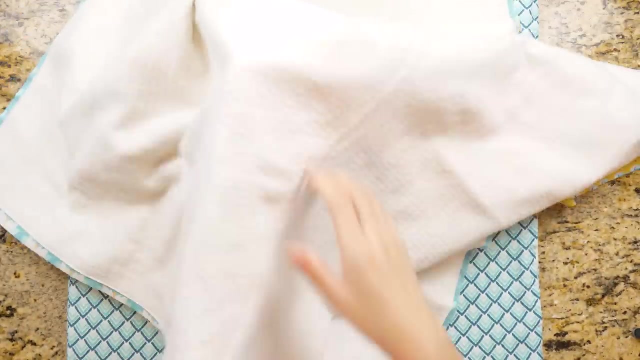 seam allowance and place a quilting ruler over the edge like this: Cut off the batting with a rotary cutter. Clip all four corners to eliminate bulk. For a neater finish, press back the seam allowance at the opening. Now start turning the blanket right-side out. You may have to manhandle it a bit. 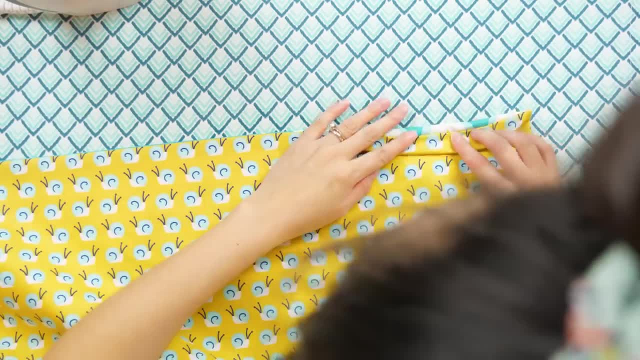 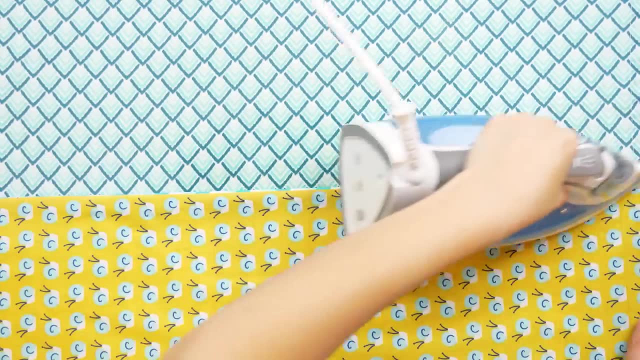 Push out the seams on each side, the best you can then press. Use an object like a child's purse to set it in place. Do this like you would, 황당, and you'll know how to sew. The sewing machine is designed for a simple, quick and fast process. 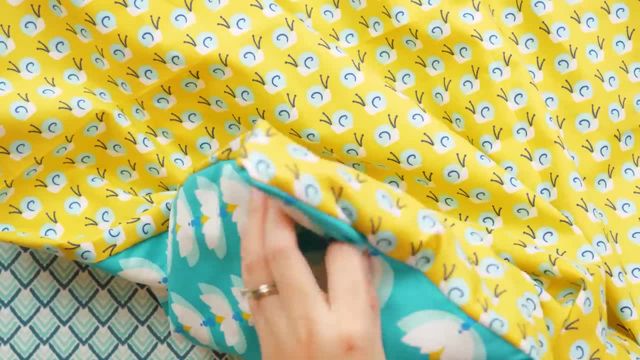 Start turning the blanket right-side out. You may have to manhandle it a bit. Push out the seams on each side, the best you can then press. Use an object like a child's purse. Do this like you would a child's purse. 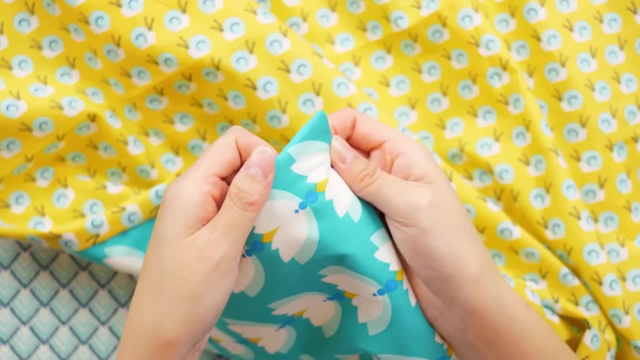 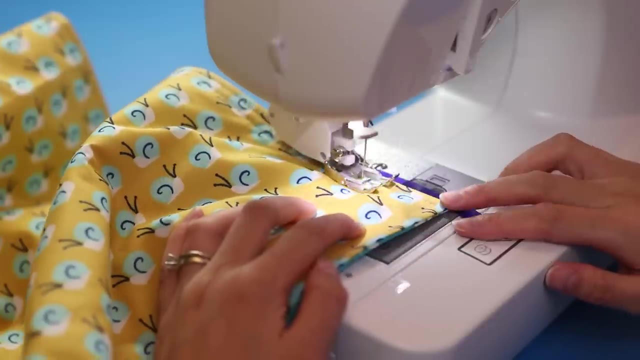 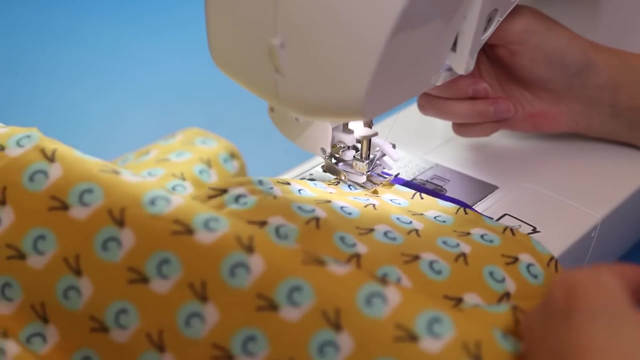 chopstick or turning tool to poke out the corners, but don't push too hard or the stitches could pop. Top stitch around the perimeter. I did two rows, one about a quarter inch and another a half inch away from the edge. I'm using a walking foot to make all of these projects because it's my favorite for most sewing tasks. 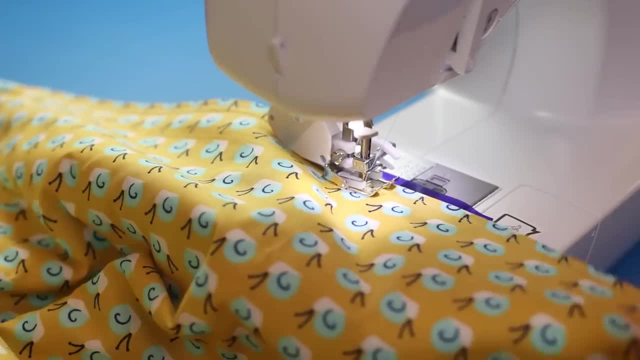 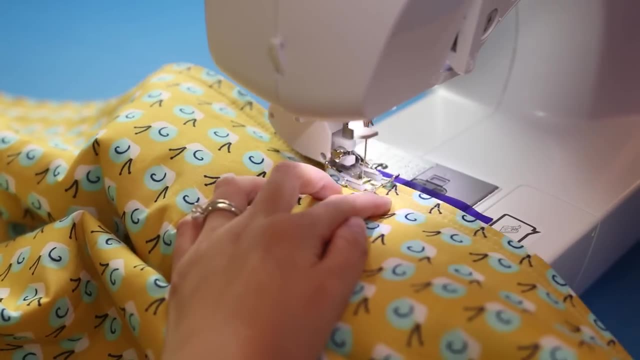 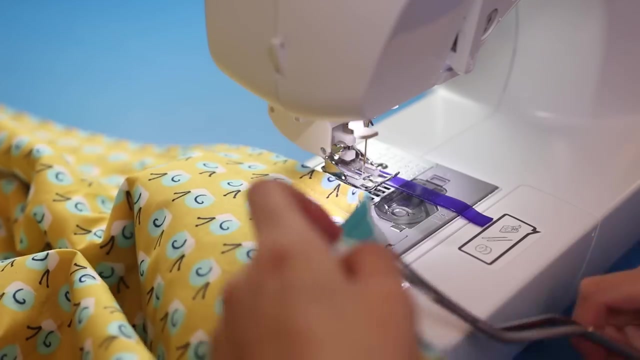 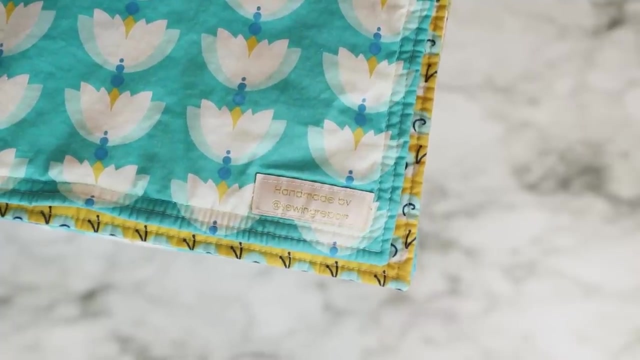 Overlap the stitches a few inches when you get to the starting point to lock the stitches. For an added touch, I included a Sewing Report Handmade label on one corner. Final measurements: approximately 35 by 40 inches- A good size for sewing. 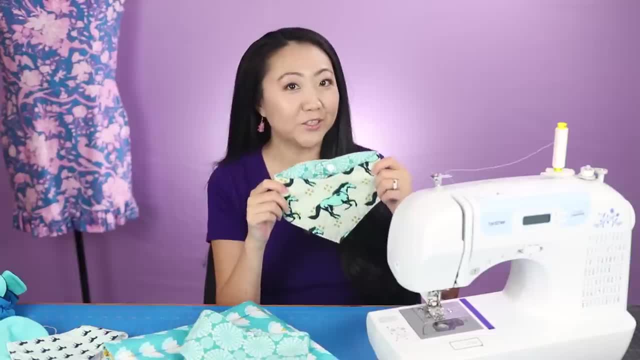 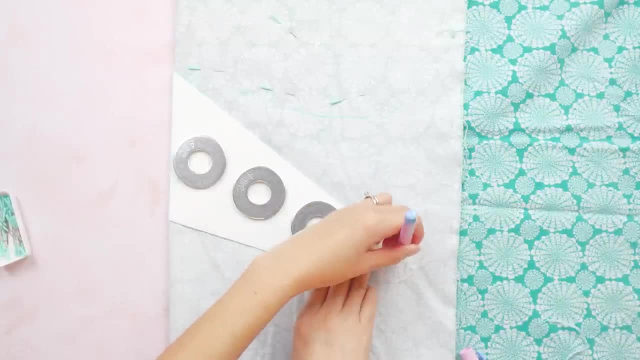 This is for a baby blanket, but you can make this in any size. Next up these great baby bandanas, Perfect for mealtimes or just a fashion accessory. This pattern is easy to follow and make. I traced the piece onto heavy stabilizer to reuse again. 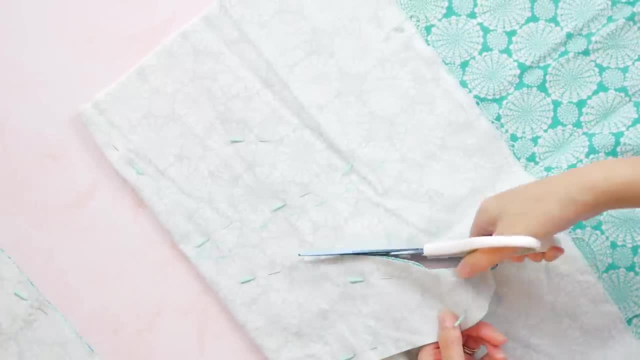 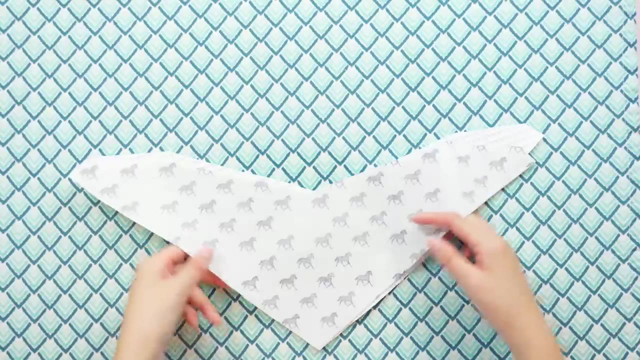 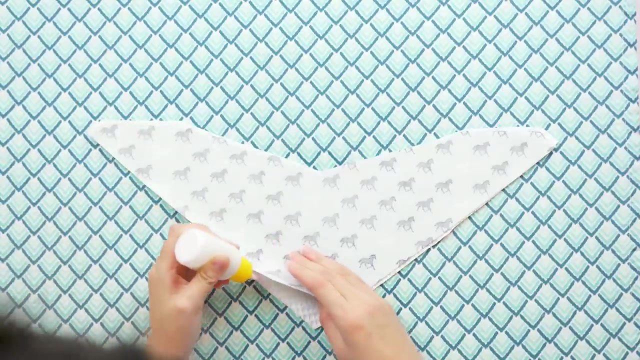 I mixed and matched prints and fabric types, including quilting, cotton, flannel and waffle weave, terry cloth Trace and cut front and back pieces, Place them right sides together. Instead of pins, I glue, basted the seams with Elmer's Washable School Glue and a hot dry iron. 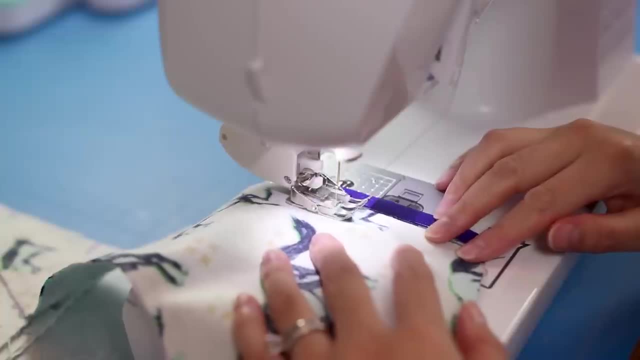 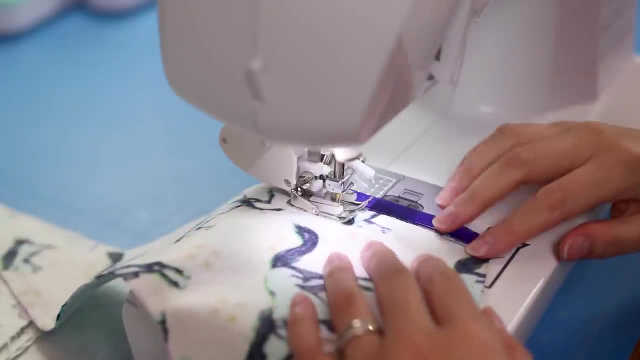 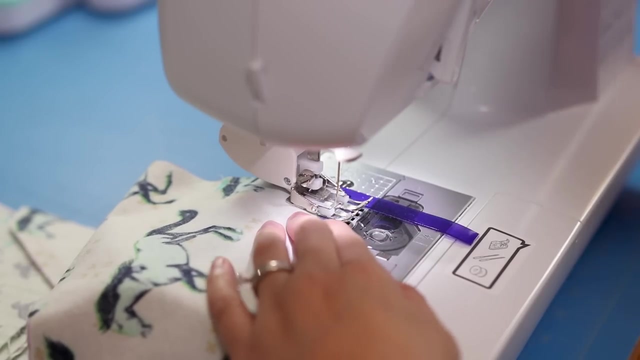 Leave a gap open of about four inches for turning. later Take it to the sewing machine and stitch around the perimeter, except for the opening, with a quarter inch seam allowance. Be sure to backstitch at the beginning and end. One tip with the walking foot is that you don't have to sew all the way to the end. If you do, you don't have to sew all the way to the end. 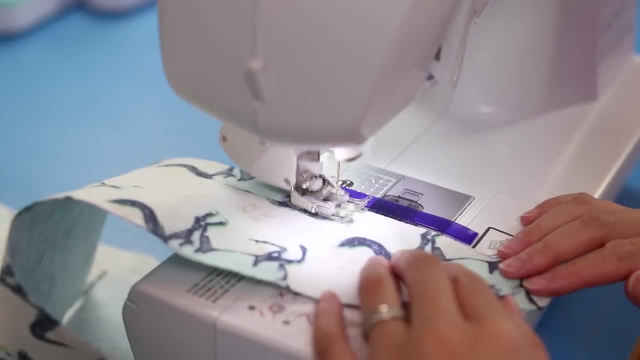 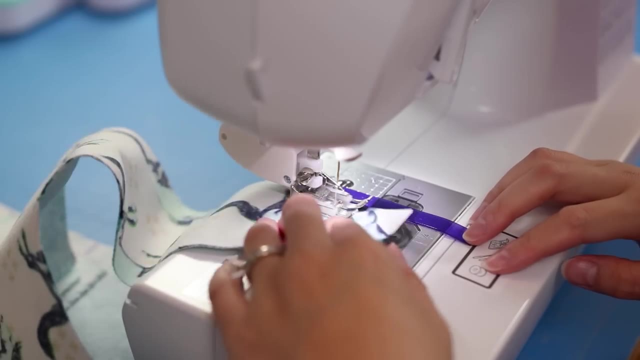 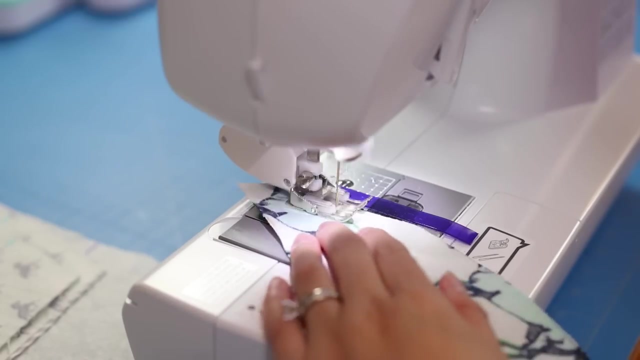 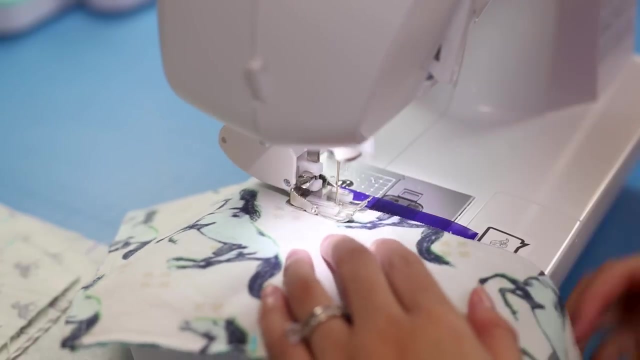 When you're doing the walking foot. if your needle position is at 3.0 and you line up the edge of your fabric at the inside metal guide, that's right at a quarter inch Sew all the way up to a quarter inch seam allowance. 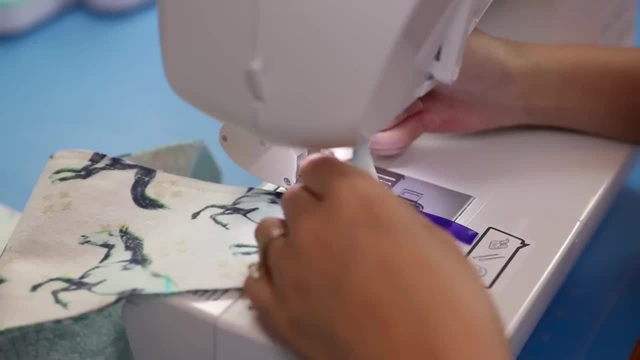 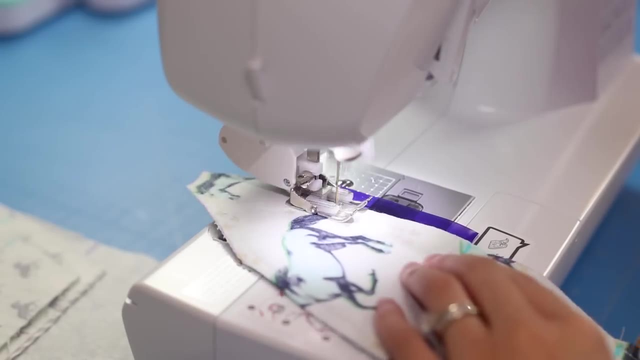 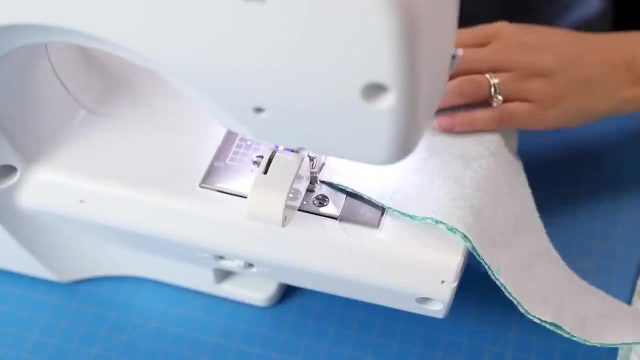 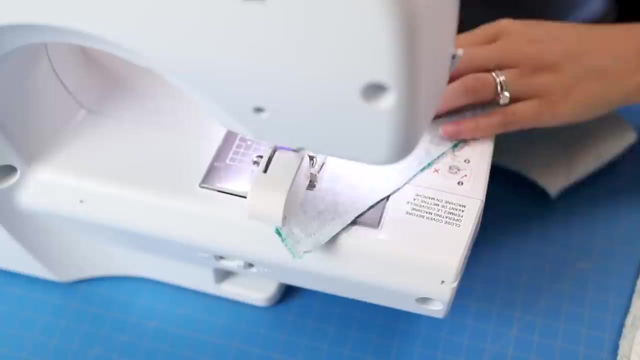 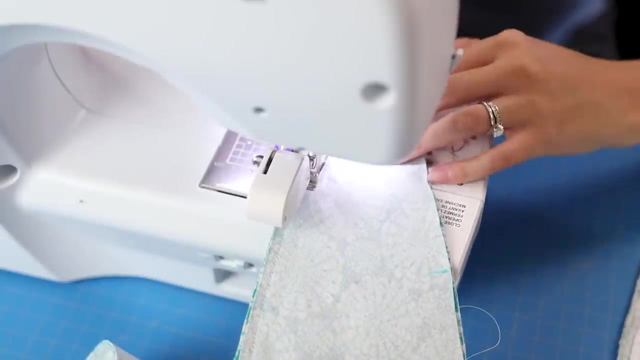 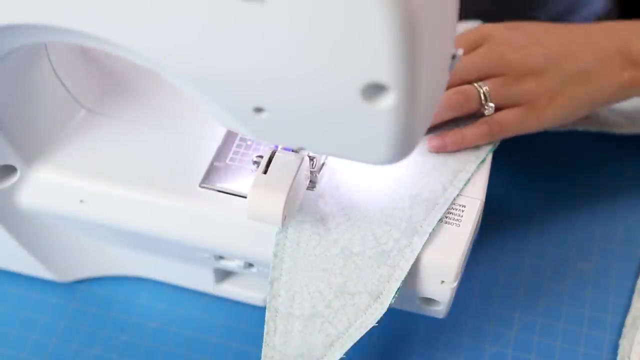 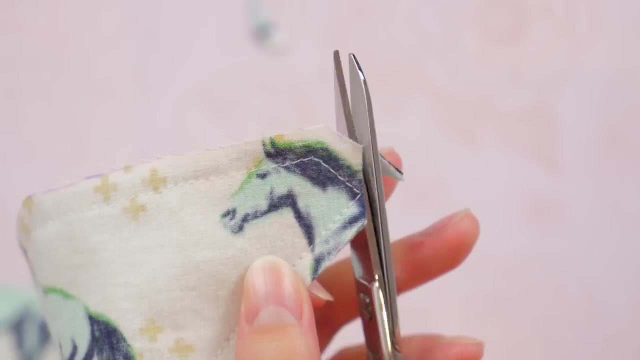 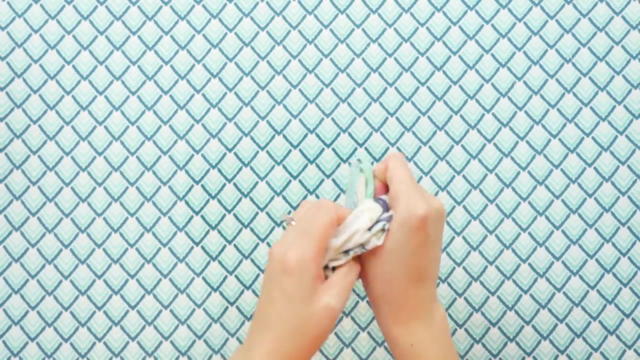 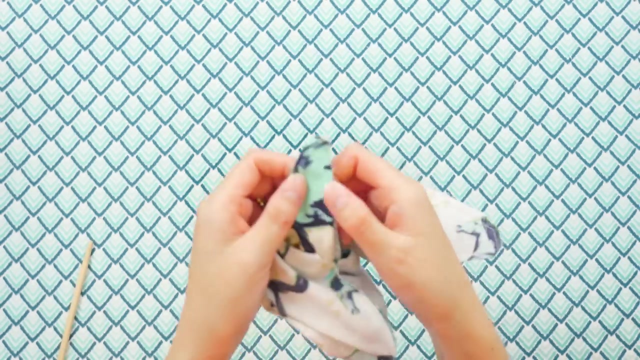 Make sure it's at 3.0. Like, and we'll see you next time. Bye, Bye, Thank you. Clip the corners to eliminate bulk Time to turn the bandana right side out through that opening. Use a point turner or a screwdriver to remove the bandana. 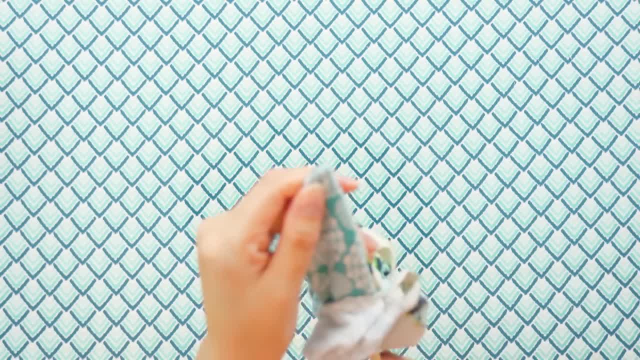 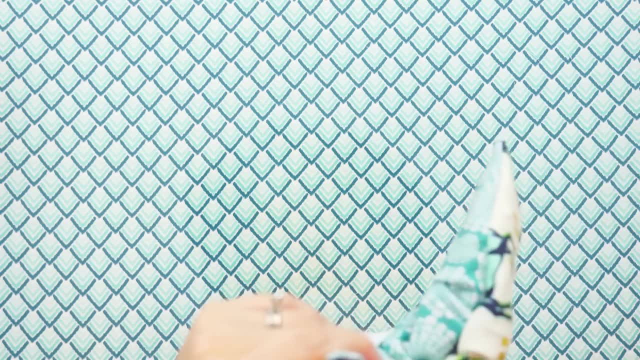 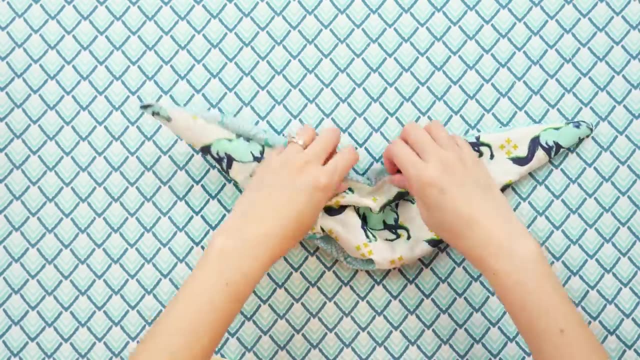 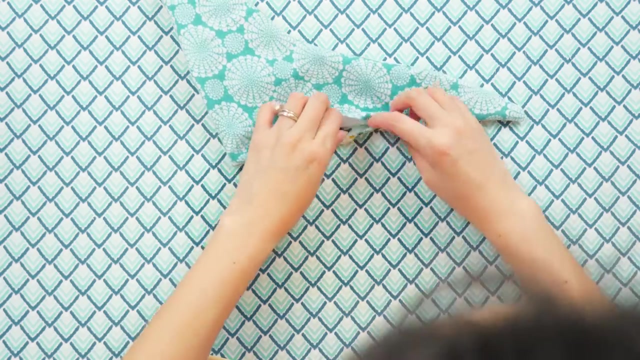 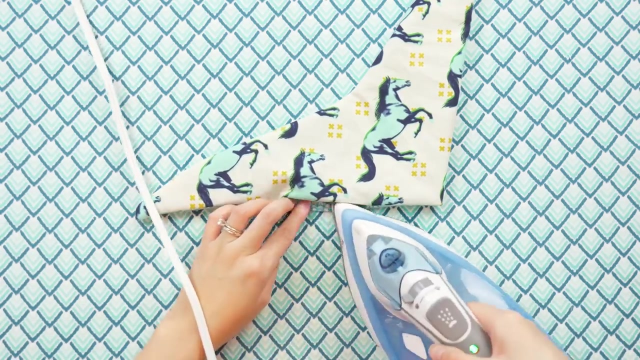 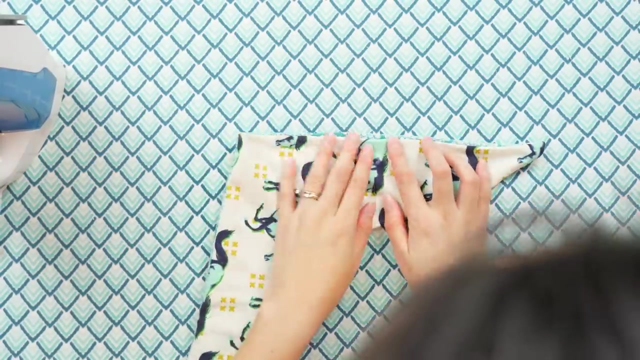 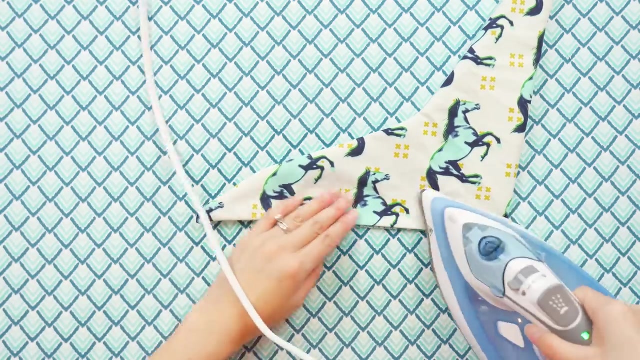 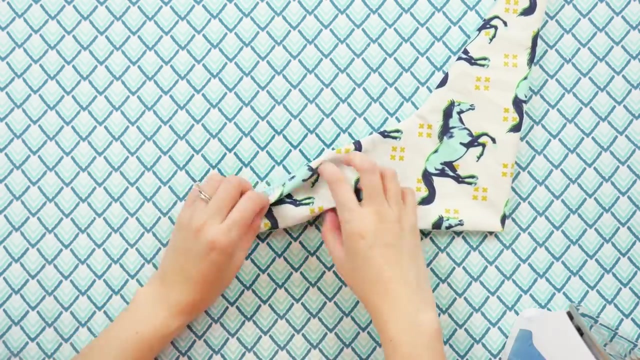 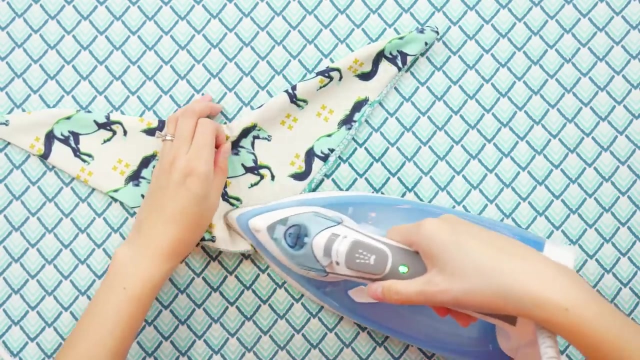 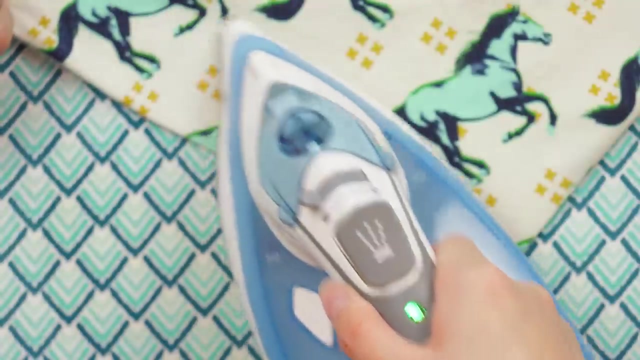 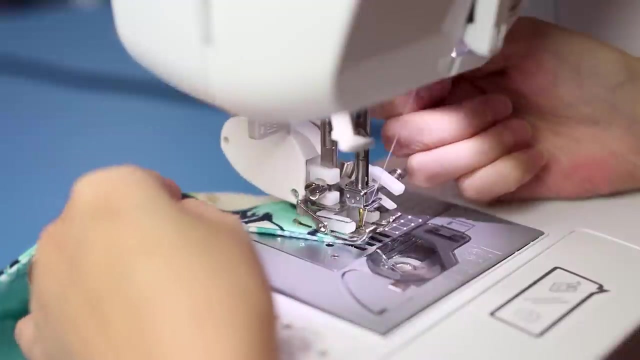 Or a chopstick to poke out the corners. Or a chopstick to poke out the corners Again. use glue to close up the opening Back at the sewing machine. top stitch close to the edge, but skip the section that will be touching the baby's neck. 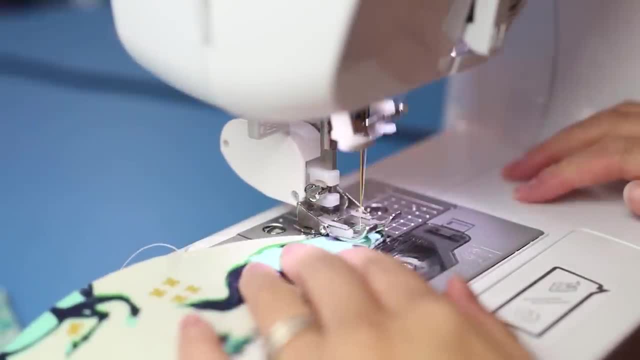 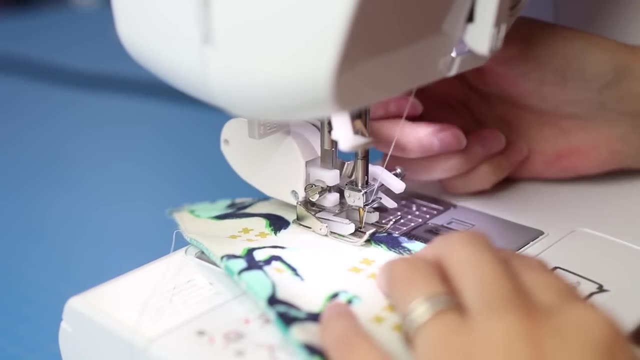 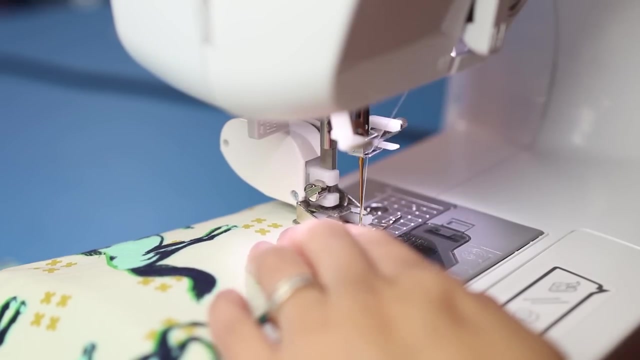 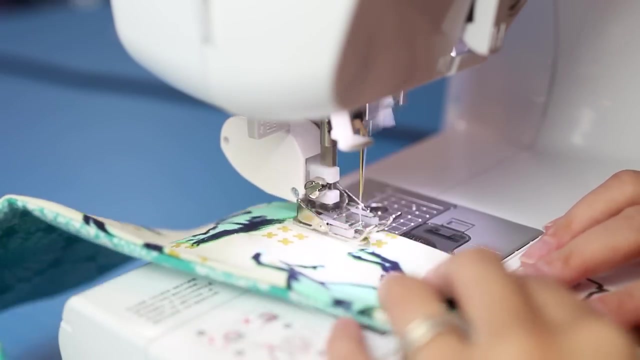 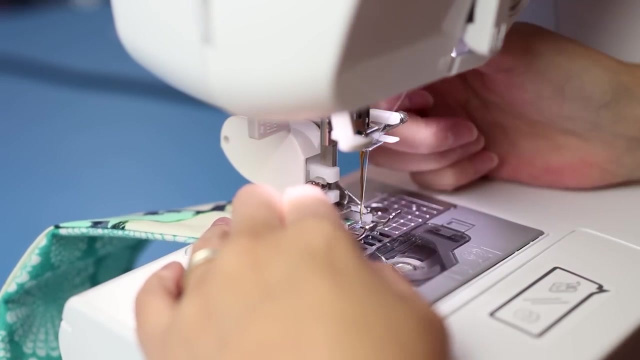 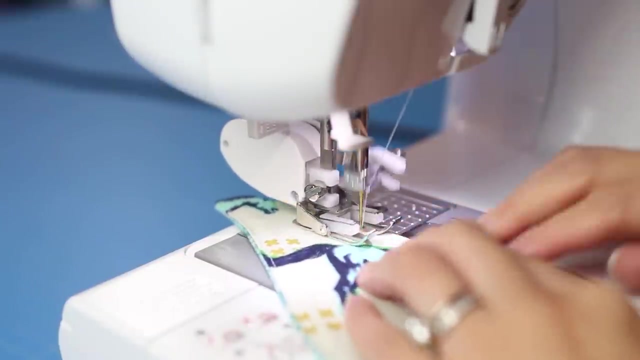 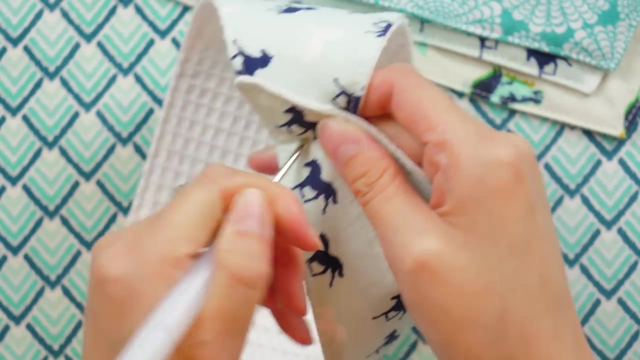 so it's softer against the skin. Back stitch at the beginning and end. The last step is adding plastic cam snaps to the ends. This is all from a kit I bought from Amazon. Poke a hole in the bandana with the included awl. 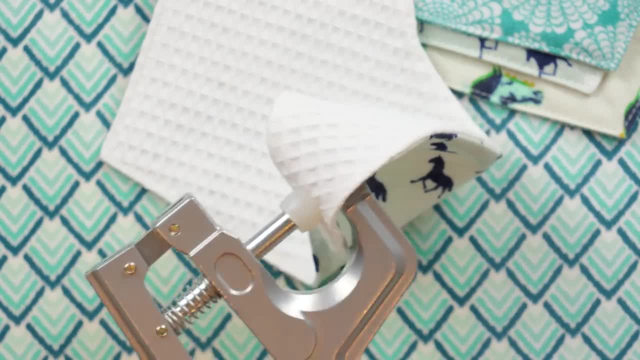 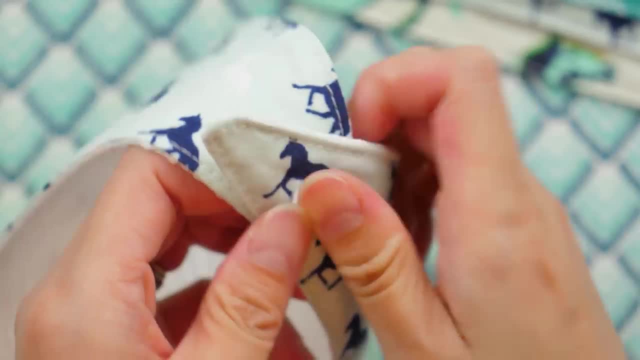 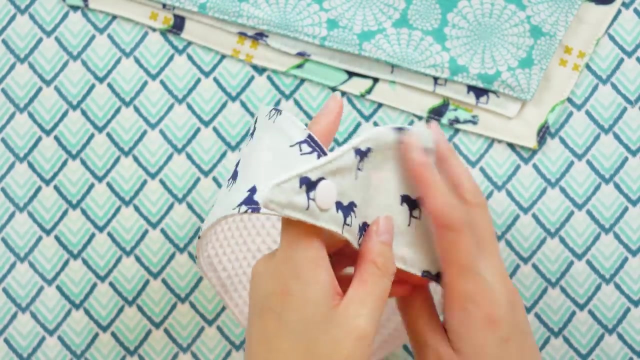 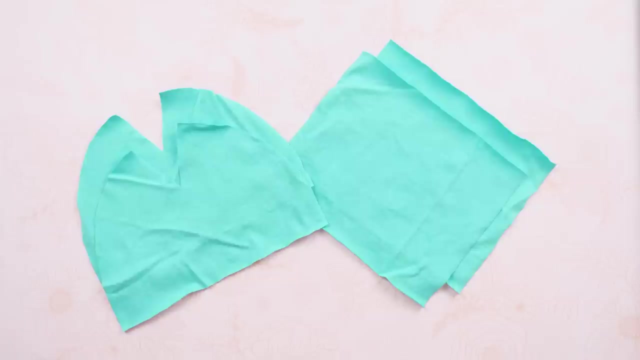 Insert the snap pieces and use the press to install them. A while back, I did a tutorial on cam snaps if you want to know more about them. These really simple knit hats are quick to make and a great scrap buster. This is a pattern I've used quite a few times. 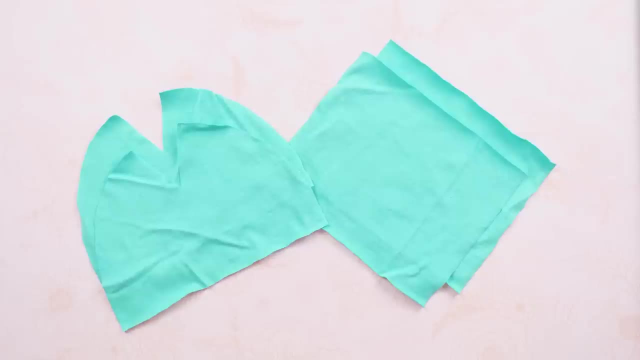 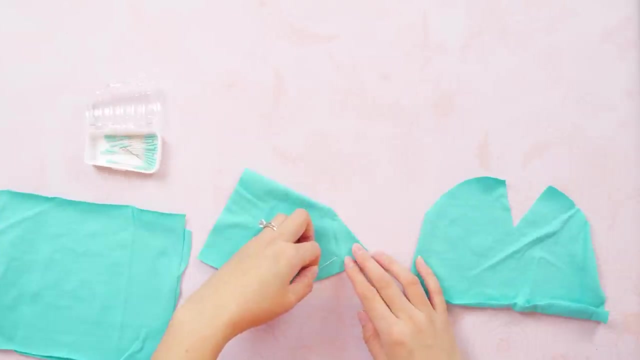 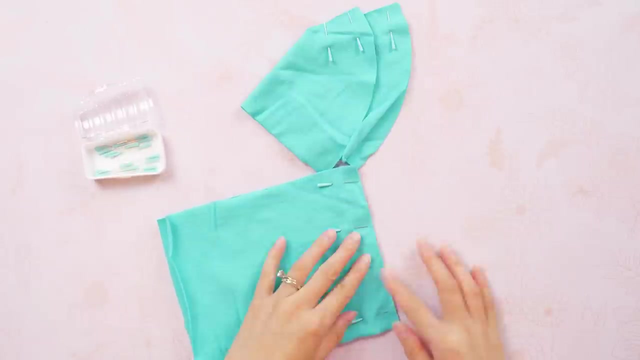 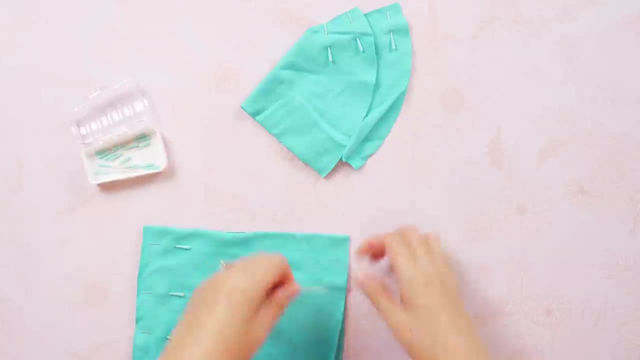 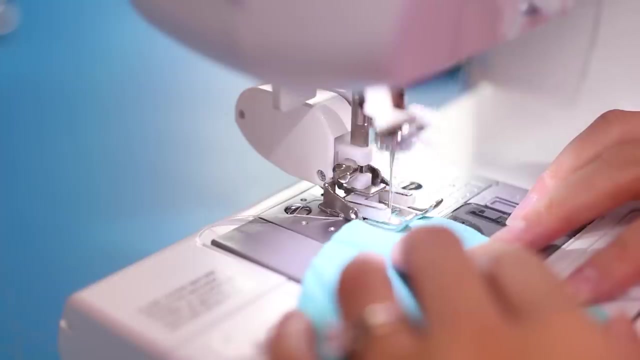 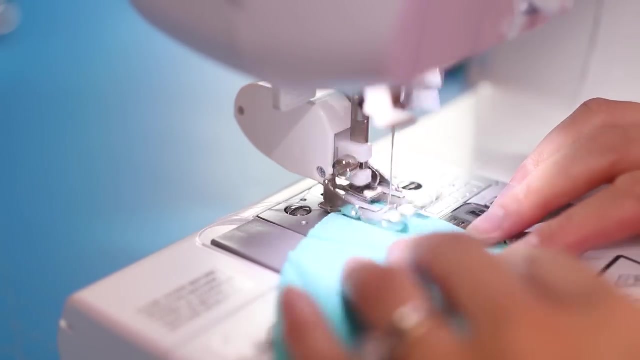 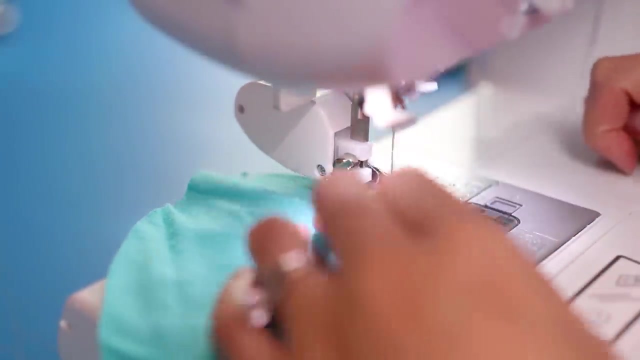 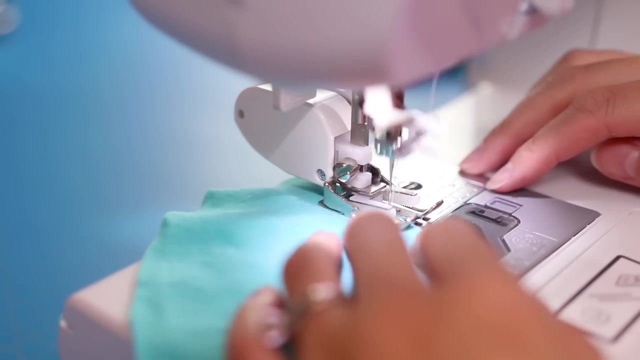 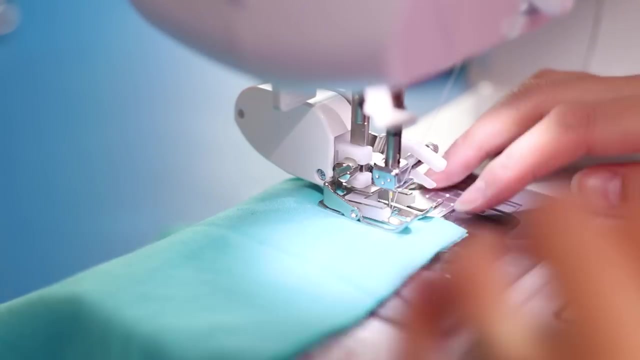 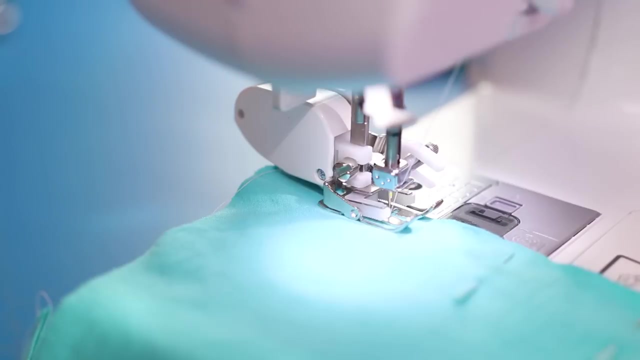 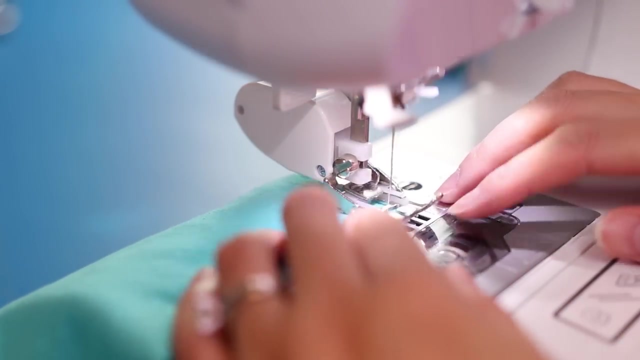 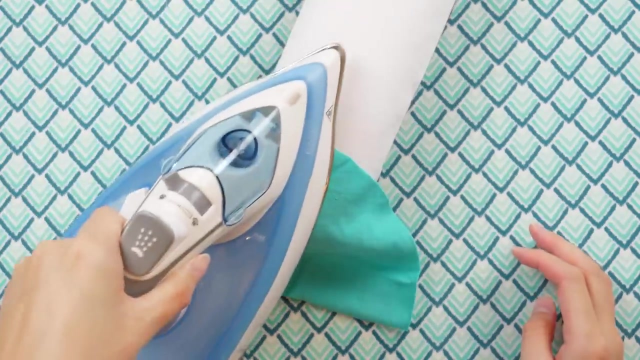 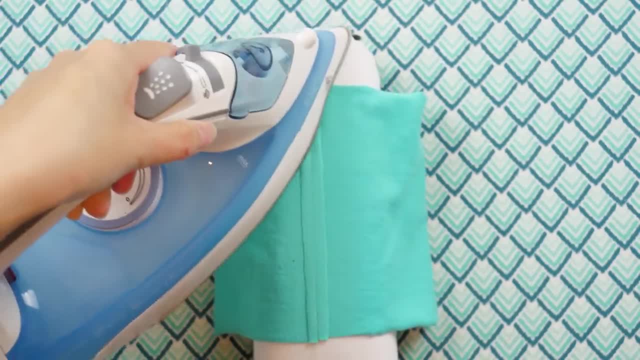 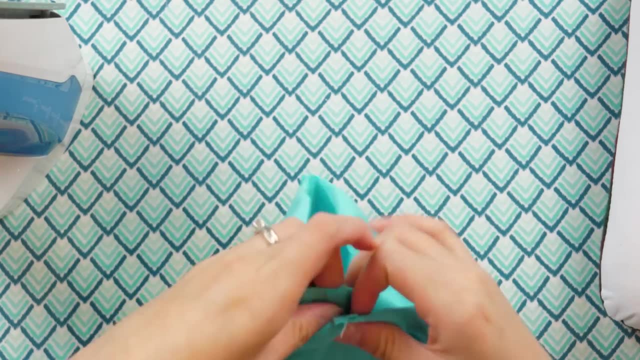 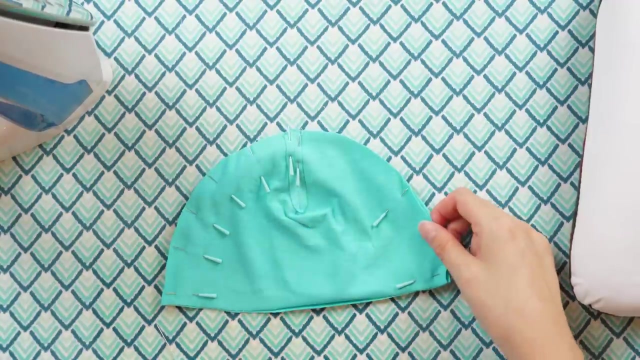 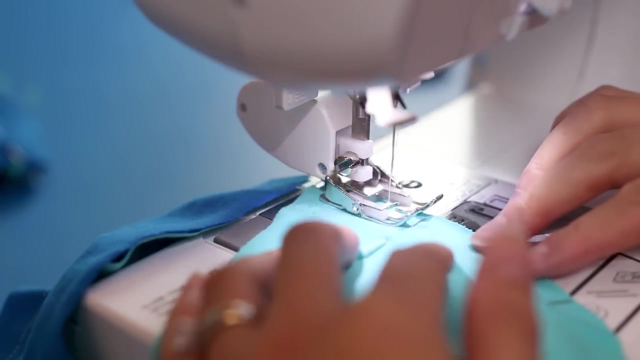 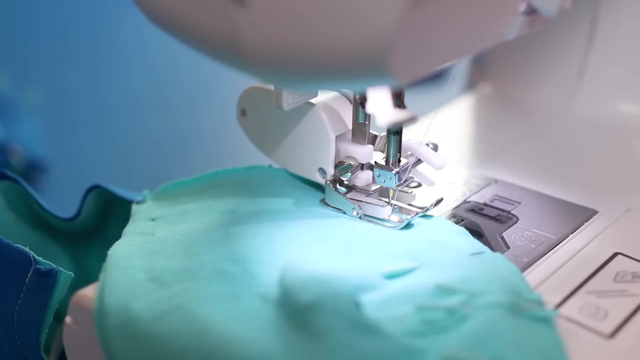 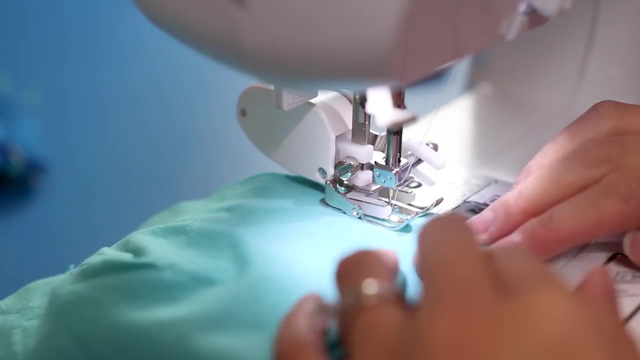 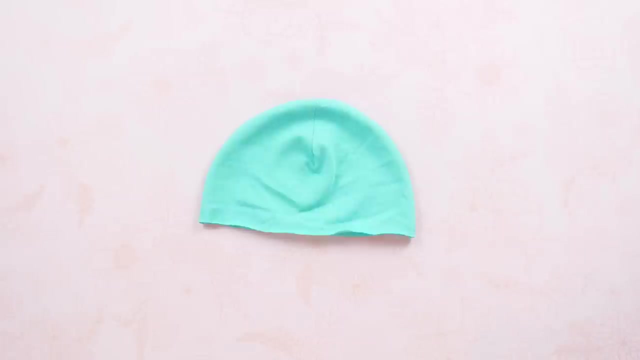 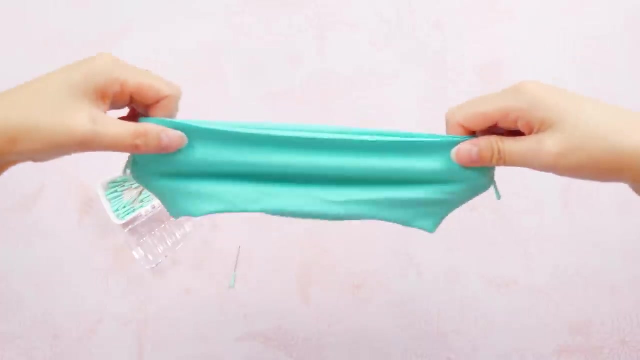 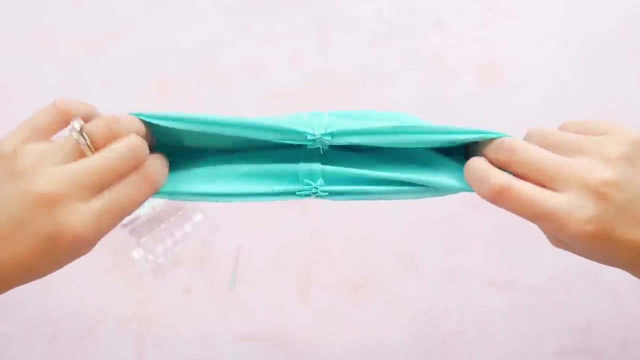 matching up the seams. fold the band, piece in half, wrong sides together. pin together the top hat pieces right sides together. so all of these with a quarter inch seam allowance right sides out, pin together the band to the top pieces. by lining up the seams the band is smaller than the hat's top when you sew them together. 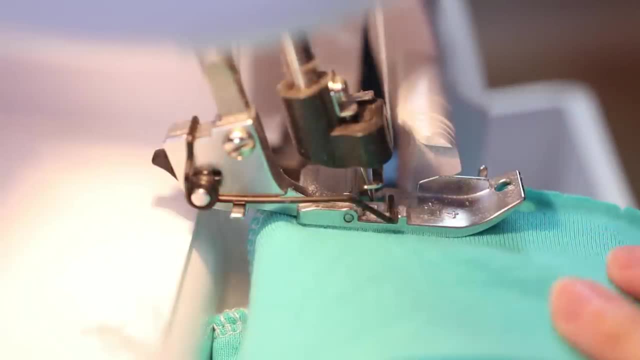 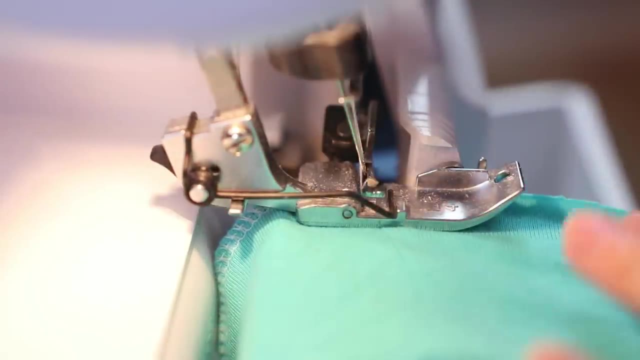 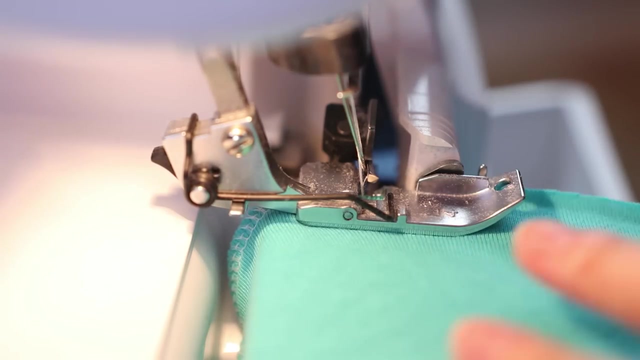 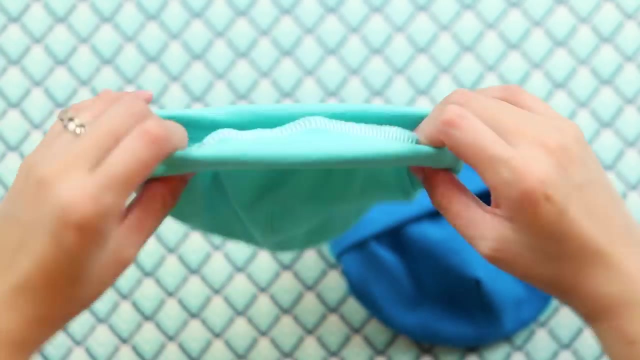 i used a serger for a cleaner finish and stretched out the band to the top pieces by lining up the seams. i stretched out the band as i went along, so the two pieces matched up. what an easy and fast project. these are the finished baby hats, with the band folded up. 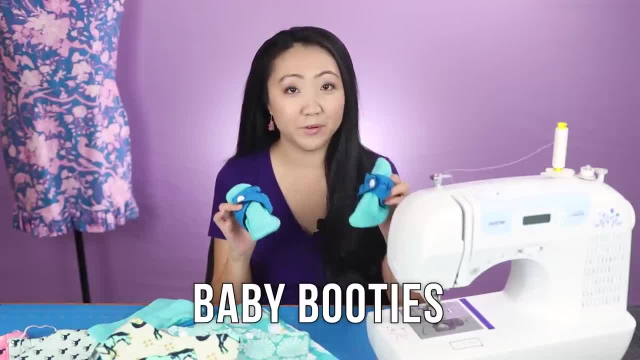 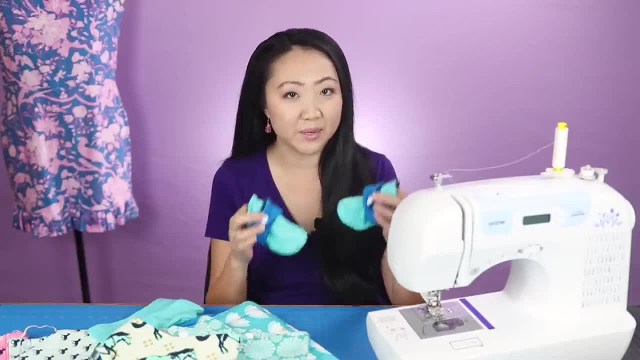 ah, i still can't get over how adorable these baby booties are. this was my first time making anything like this project. there were a few steps that tripped me up and i'll explain in my demonstration what i think could make it easier. i will certainly make these. 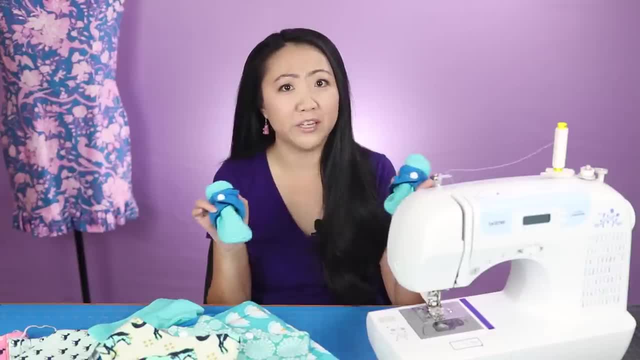 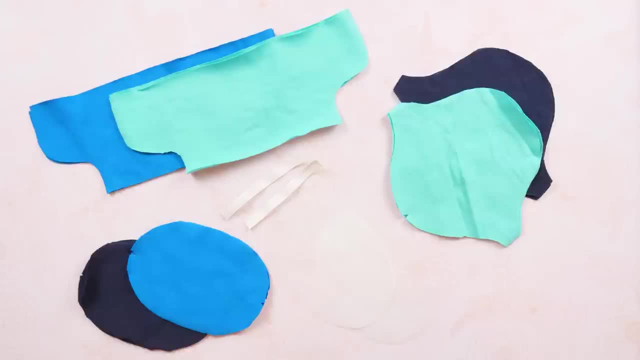 again. i think they turned out just adorably freaking cute. here are all the cut pattern pieces laid out. plus the elastic, they make one pair of booties. this was probably the most difficult project out of all of them, but i learned a few tricks. first, prepare some of the pieces: place. 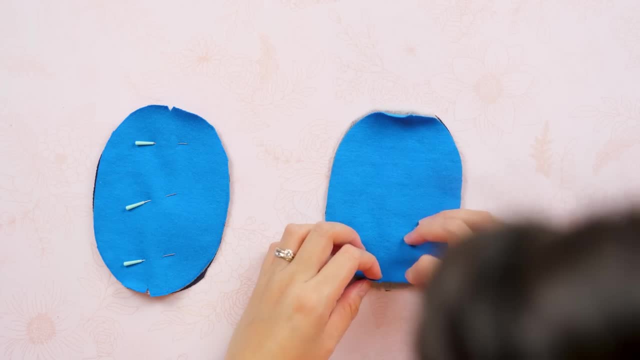 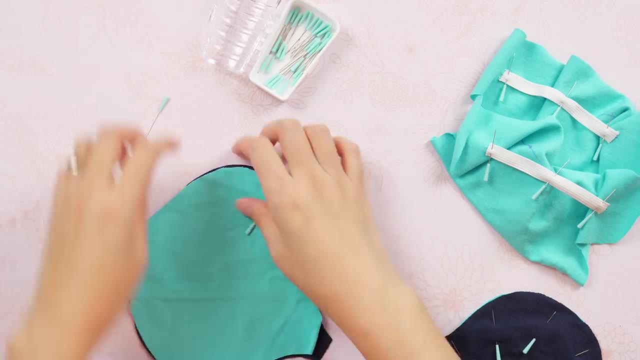 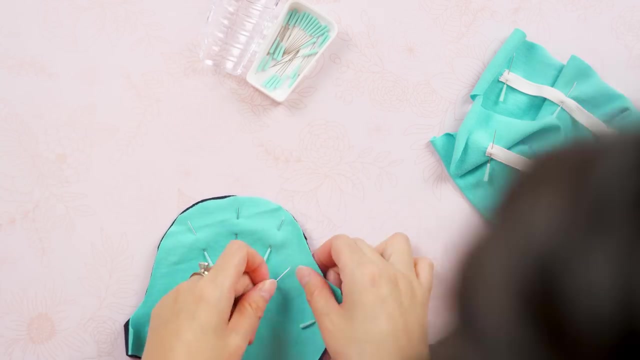 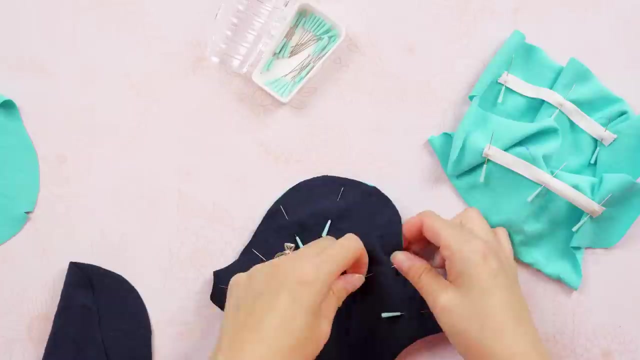 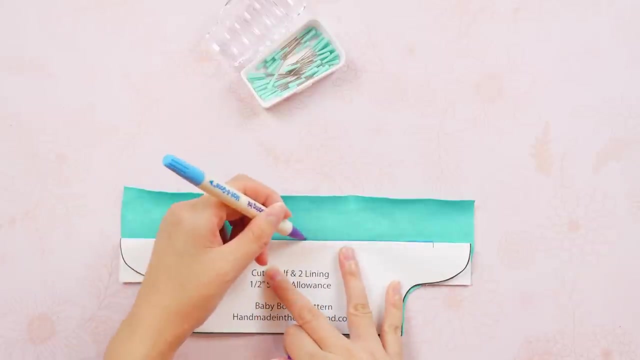 the bottom sole pieces wrong sides together and then fold them in half to make a pair of booties and then sandwich a layer of sew-in interfacing in between. pin all three layers together. right sides together. pin the tongue pieces. the back piece was the most difficult to instruct because it requires stretching elastic over it. 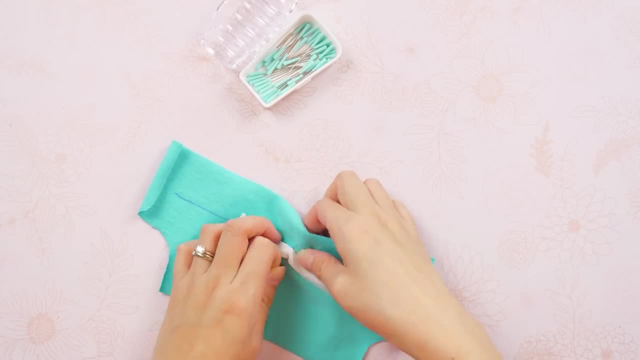 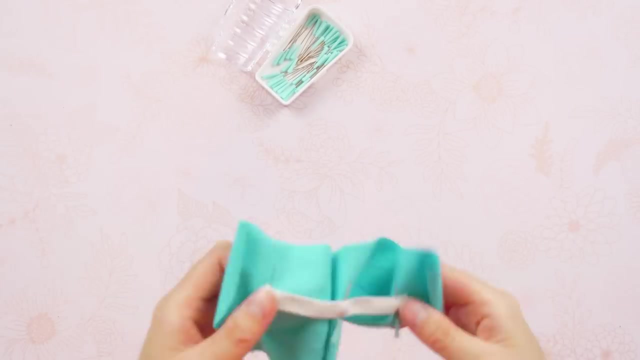 well and tight, so i decided to make a pair of booties that are just as tight as possible and while sewing at the same time. originally, i followed the instructions with a three and a half inch cut of elastic pinned at the ends and middle of the marked line. this did not work well. 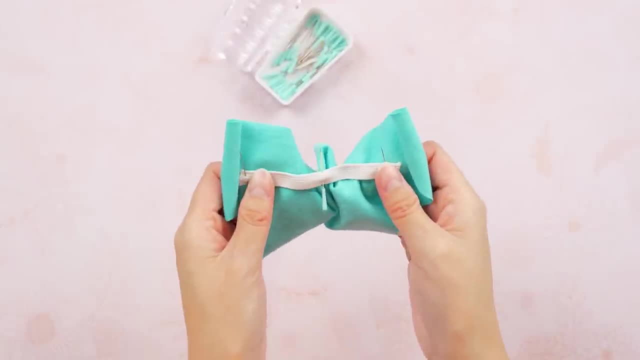 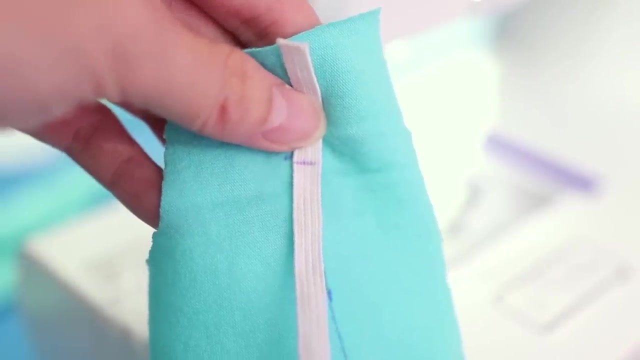 for me. instead, i cut a four and a half inch piece and marked out the three and a half inch section. i lined up one end with the markings and placed under the sewing machine. the secret is that i started sewing a little before the marking back, stitch and stitch until the marking. 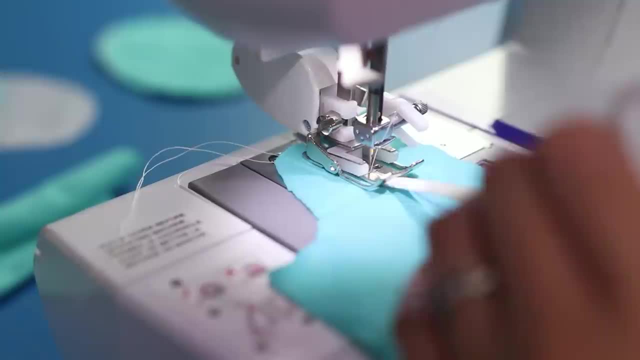 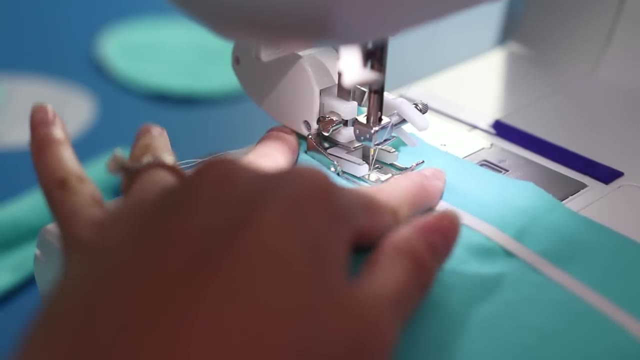 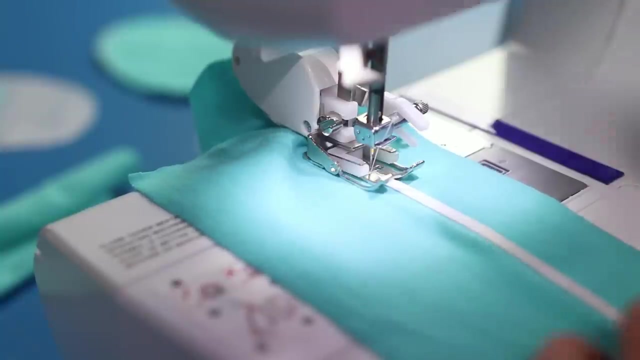 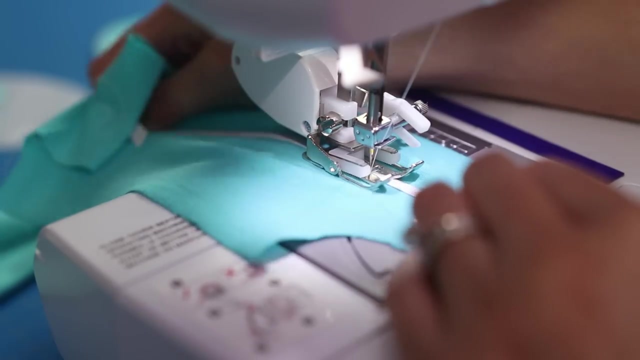 is tight. then stretch the elastic out and match up markings on the other side with one hand. using the other hand, hold on to the piece behind the presser foot and continue stitching. once you get to the end marking, make a few stitches forward and back to lock in. 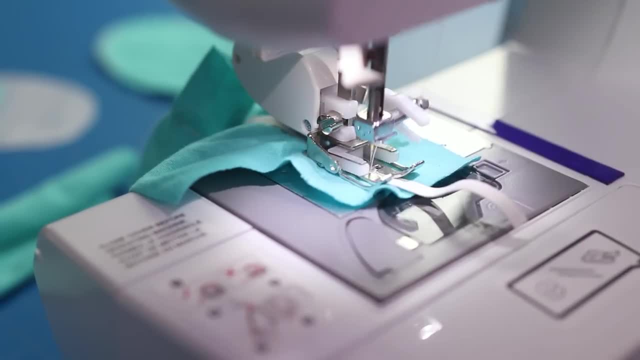 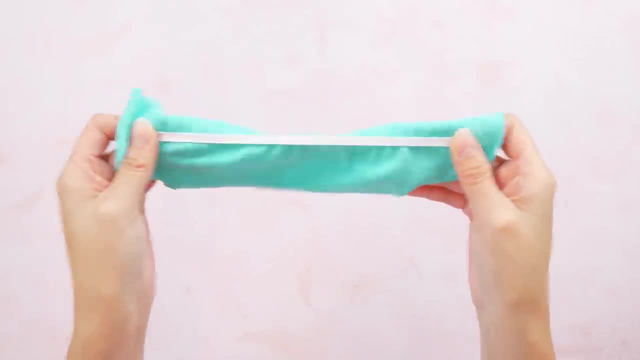 in place. After removing from the sewing machine, cut off the excess elastic- This is how it's supposed to look- and stretch. And, by the way, the elastic goes on the wrong side of the fabric. With a quarter inch or less seam allowance, sew the bottom sole layers together. 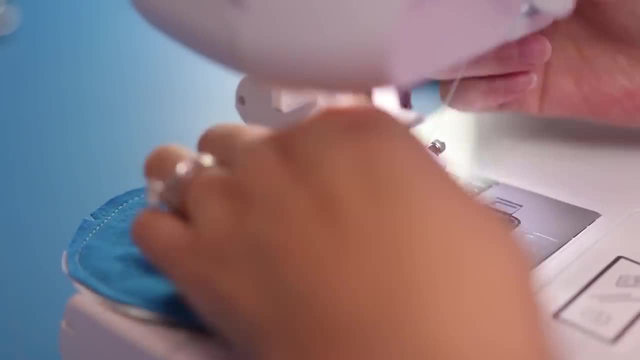 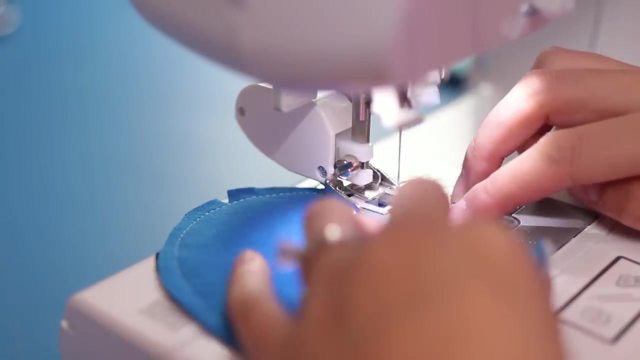 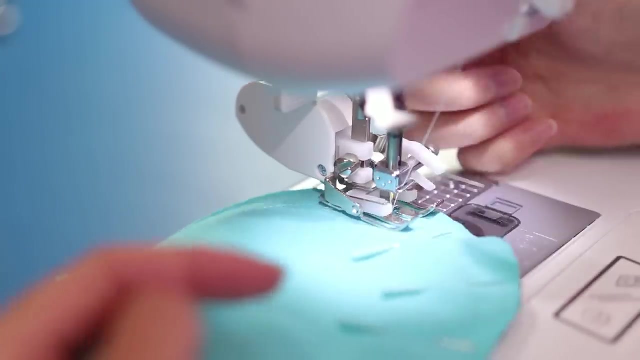 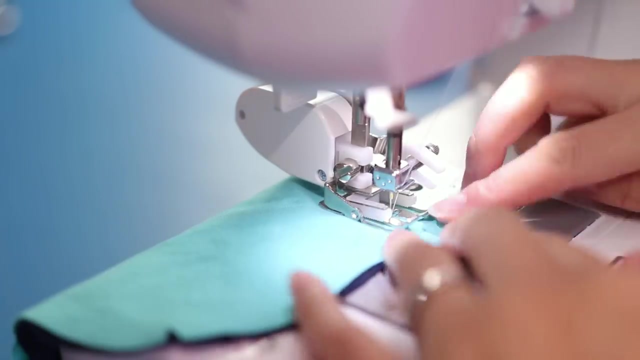 From here on out, you'll be using a half inch seam allowance. Sew the tongue pieces together, back stitching at the beginning and end. Trim the seam allowance down with scissors. Turn right side out and sew the seam allowance down with scissors. Turn right side out. 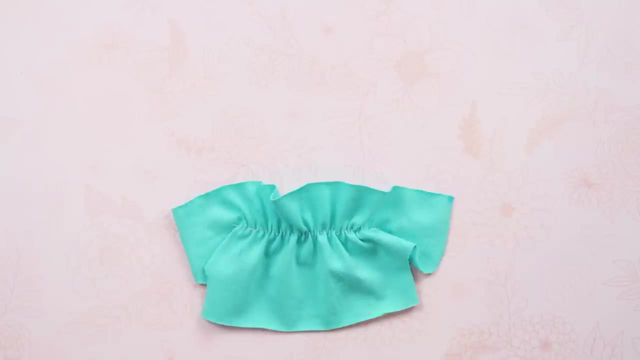 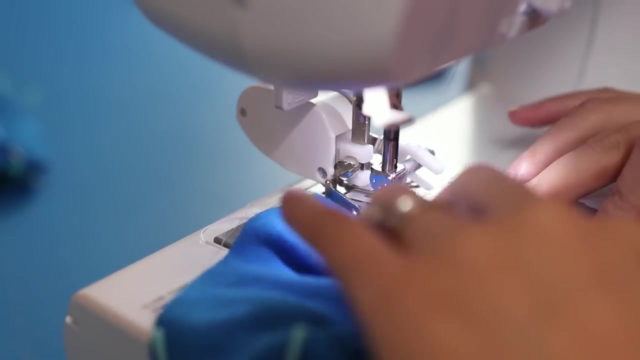 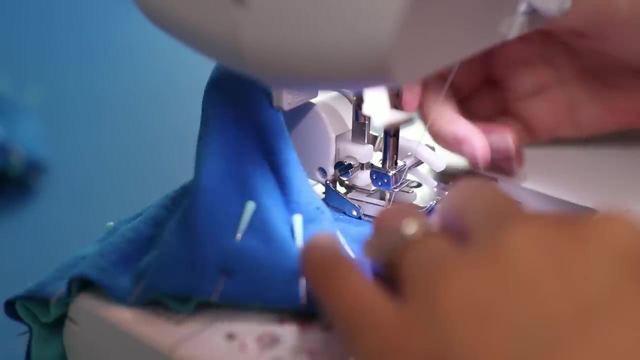 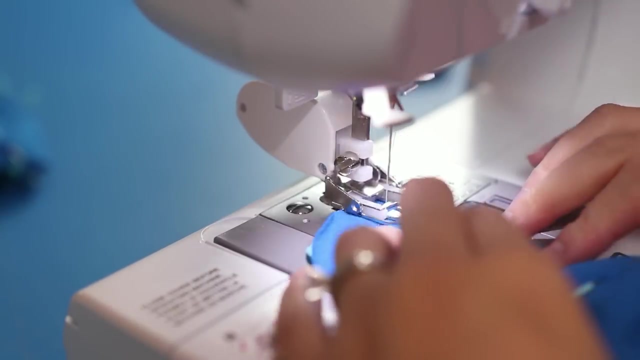 and sew the seam allowance down with scissors. Turn right side out and press. Pin together the back pieces right sides together, but leave the shorter end of the long sides open for turning. Sew together with back stitching at both ends. Be careful and go slow around those curves. Trim down the seam allowance and turn right side out. 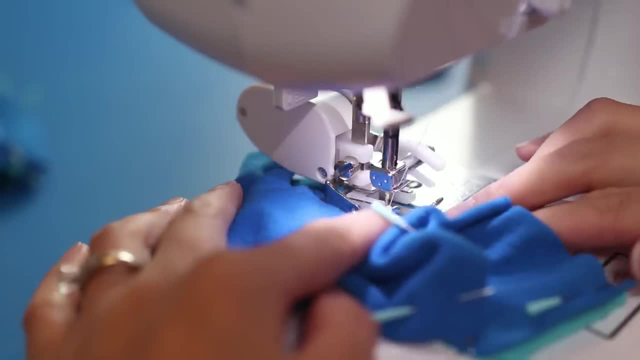 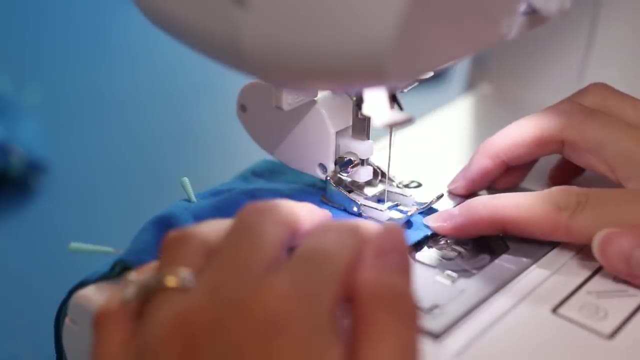 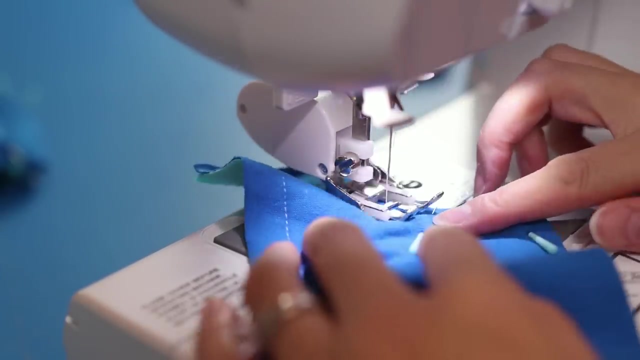 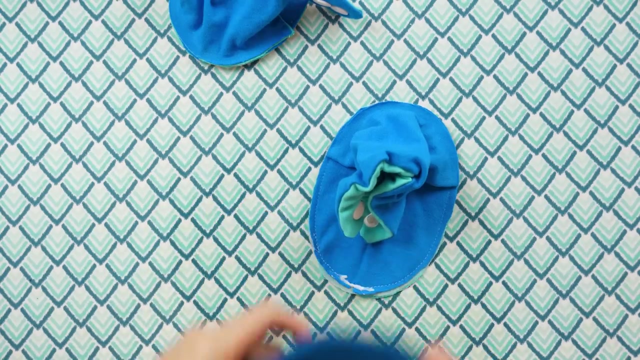 The three pieces of seam allowance together are the same as that on the front. Trim all the way around. Give the back piece of the front a little push before cutting. Sew the lining up the center notches. Secure the back and tongue pieces to the bottom with the side you want facing out on the inside. 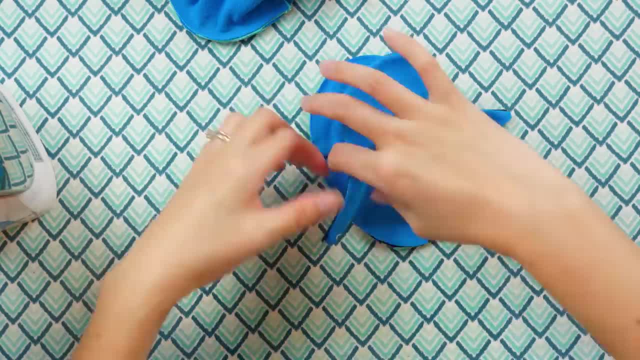 The lining up the center notches. Secure the back and tongue pieces to the bottom with the side you want facing out on the inside. You can use pins, but I used glue. You'll need to stretch the back and tongue pieces so they overlap a good amount. 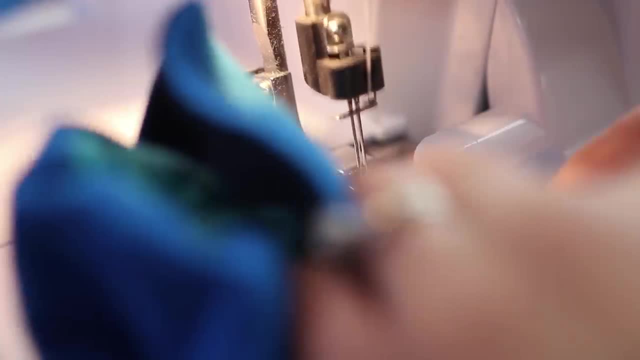 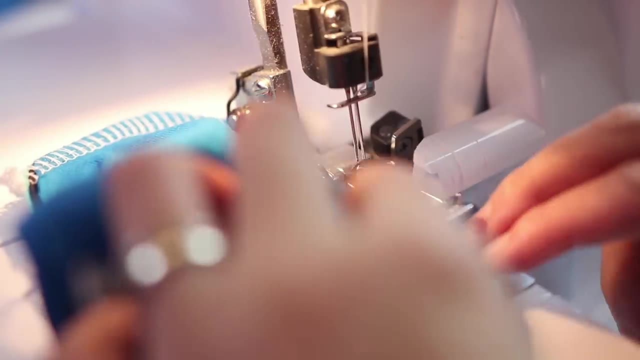 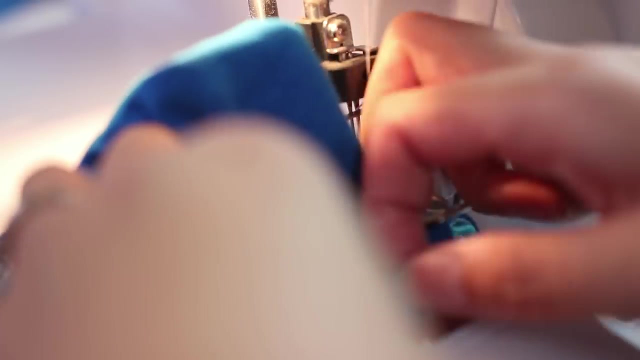 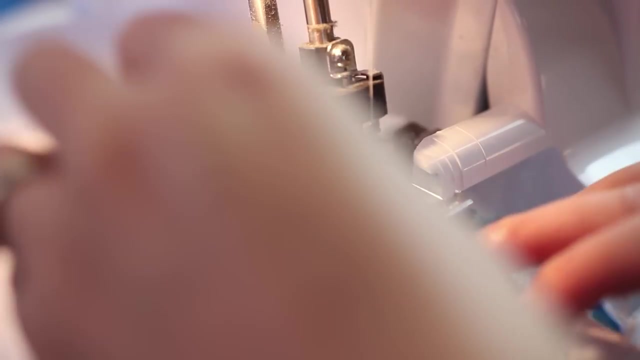 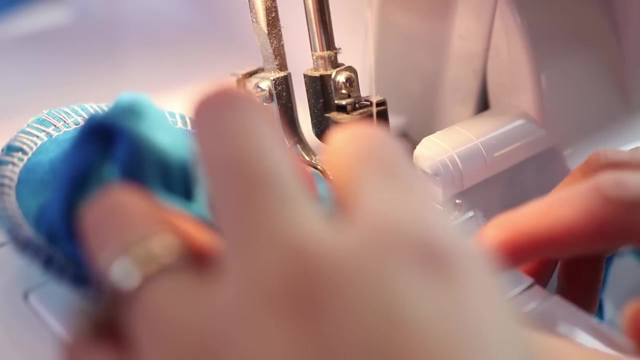 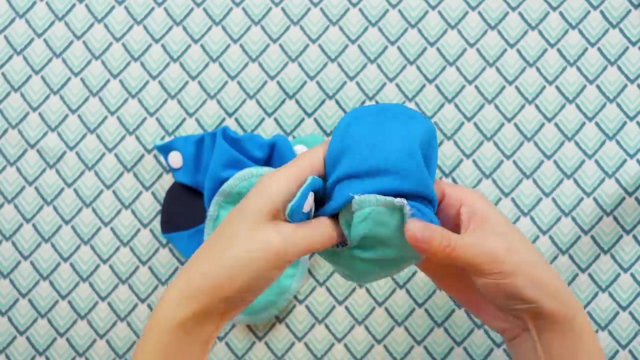 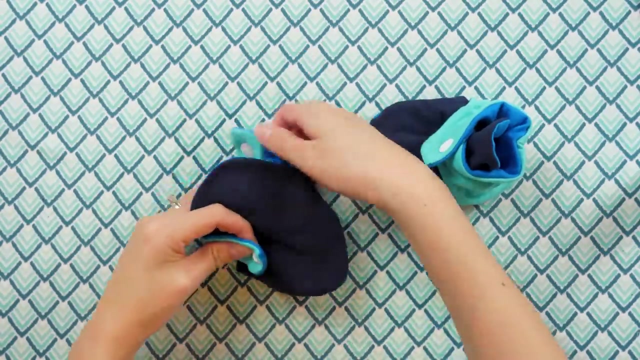 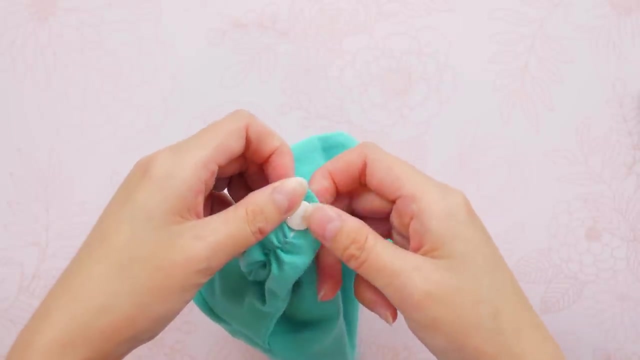 Sew or serge all around the boot sole. Turn the booties right side out. Now to add cam snaps to the tabs. Poke a hole in the bootie with the included awl, Insert the snap pieces and use the press to install them. 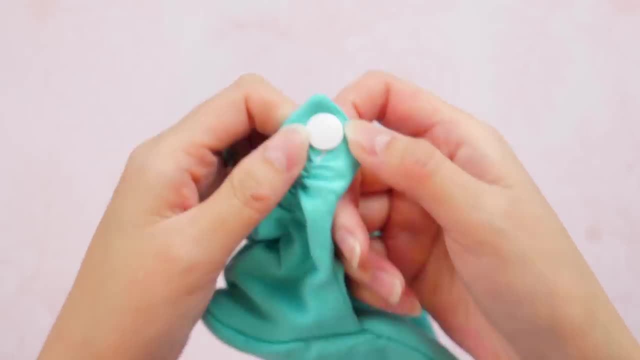 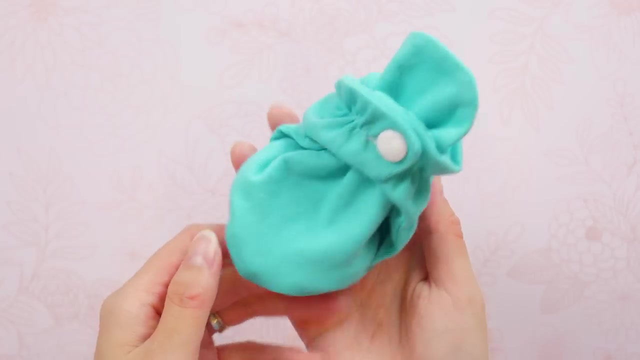 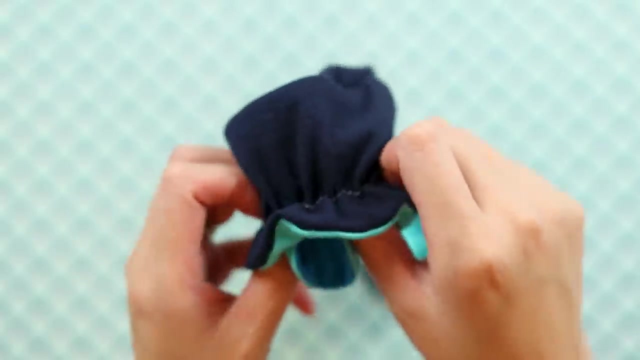 And again, be sure to check out that more in-depth video I did on installing cam snaps. Here are the finished baby booties- Without question the most time-consuming but very satisfying to finish. Burp cloths are a fantastic go-to baby gift. 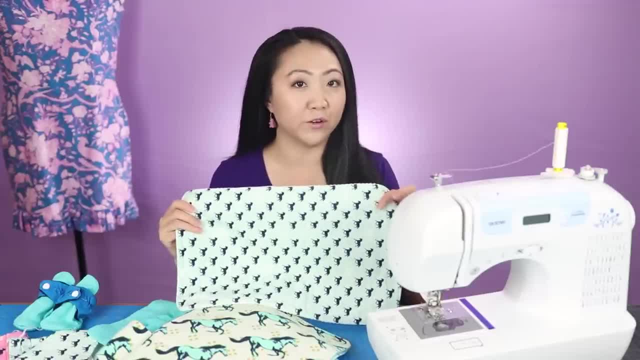 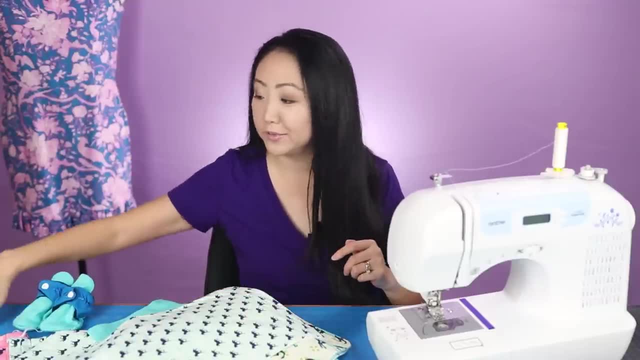 New moms love them. I've gotten a lot of great feedback over the years from burp cloths I've given friends And I've tried a few different patterns, but for this one I wanted to make my own, So available now on SewingReportcom. 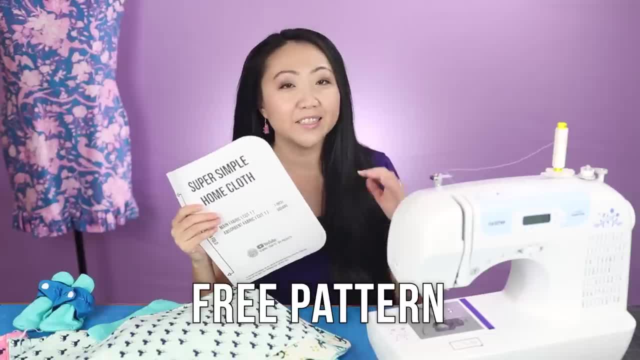 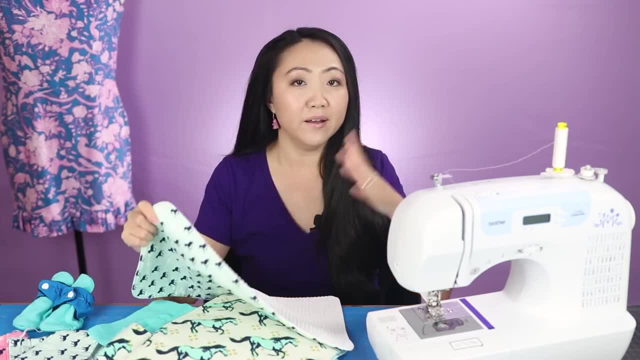 My pattern for super simple home cloths, And I didn't call the pattern burp cloths because I feel like these could have quite a few different uses. Obviously, I'm not a fan of burp cloths, but I've tried a few different ways. 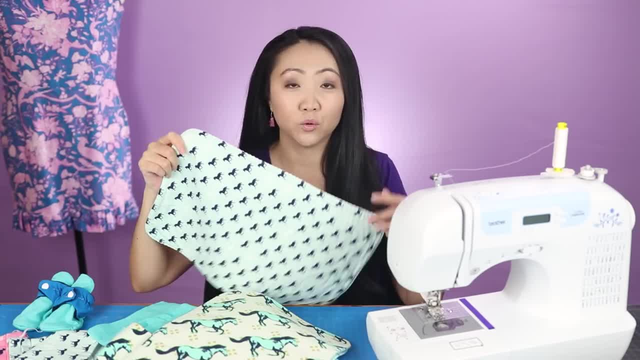 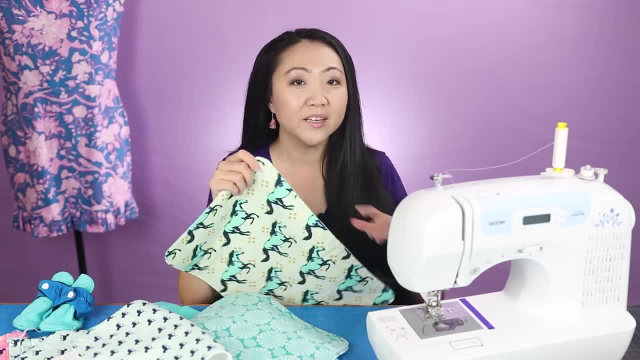 So I'm going to show you how to do different ones. Obviously now there's kind of a paper product shortage, so you could use these as reusable paper towels, just everyday cleaning place mats, Depending on what type of fabrics you use. 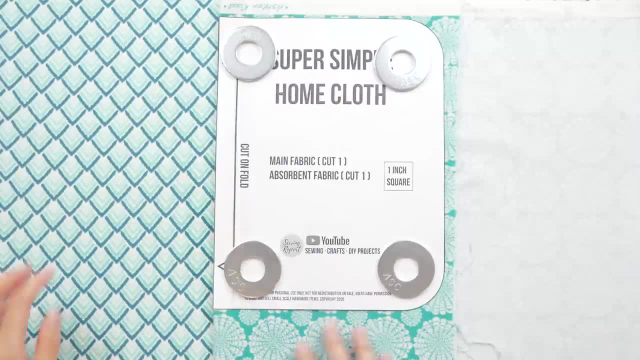 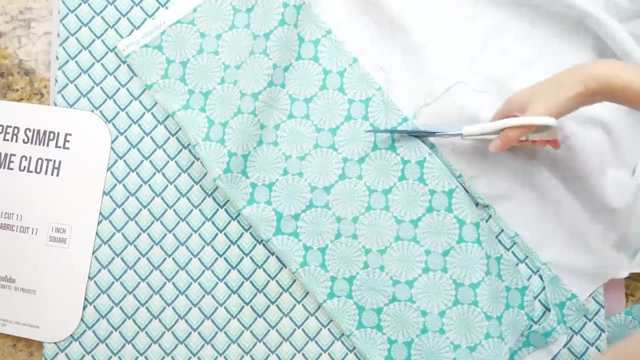 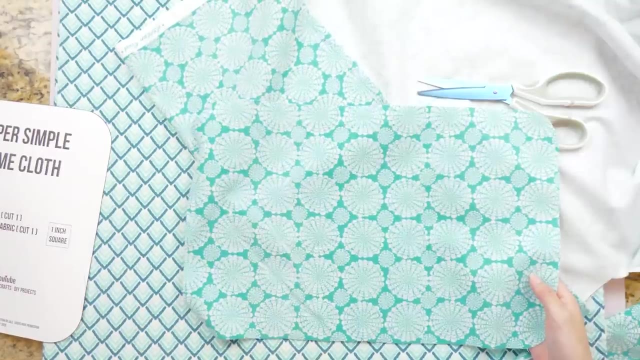 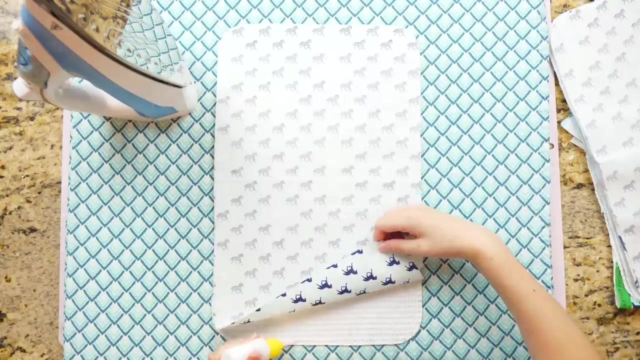 these cloths can have all different sorts of functions: around the house or with a new baby. Download and print out the pattern It's meant to be traced and cut on the fold. Place the pieces right sides together. I typically do one side as quilting cotton and the other more absorbent fabric like flannel. 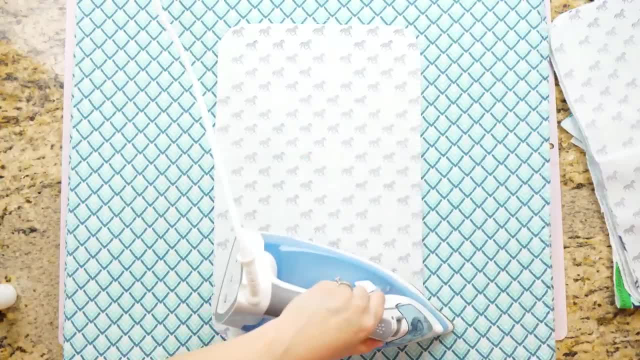 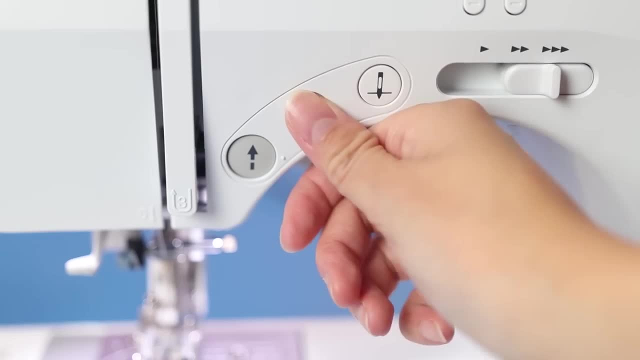 or terrycloth Instead of pins glue. baste the seams with Elmer's Washable School Glue and a hot dry iron. Leave a gap open of about 4 inches on one side for turning later At the sewing machine. stitch around the perimeter with a half inch seam allowance. 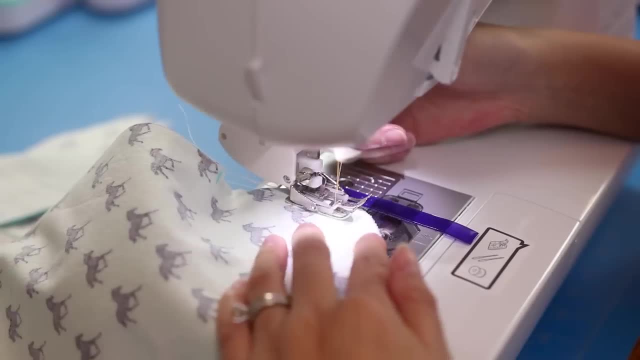 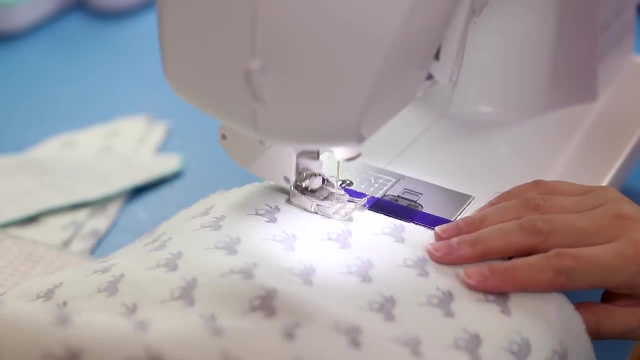 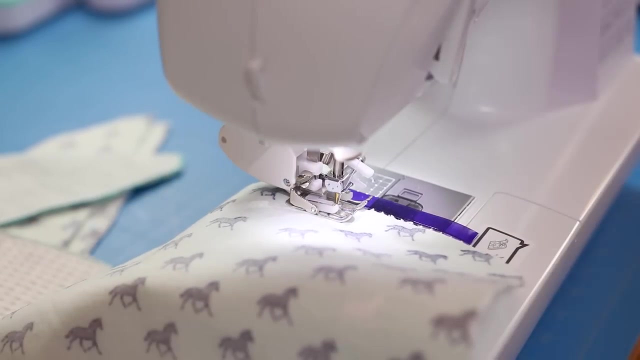 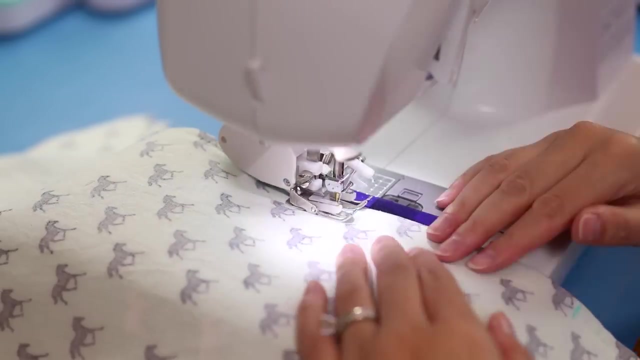 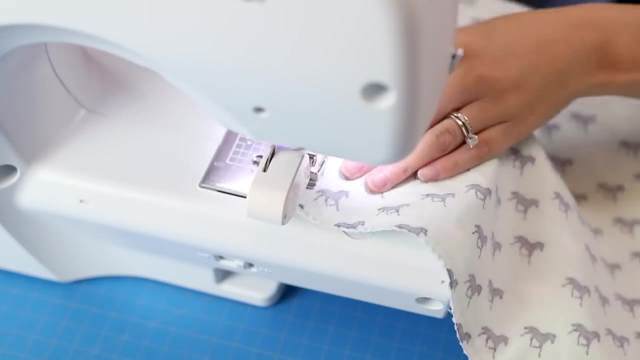 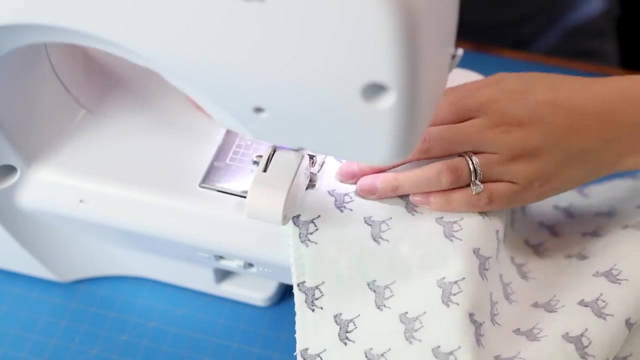 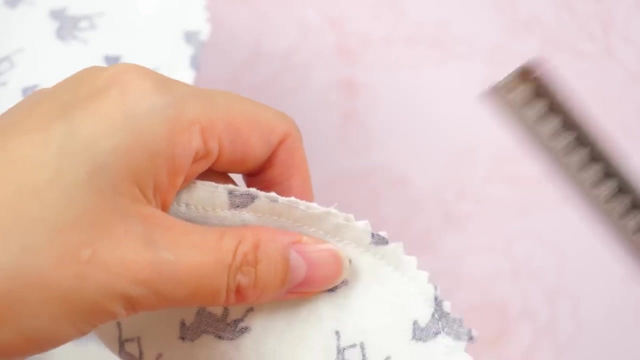 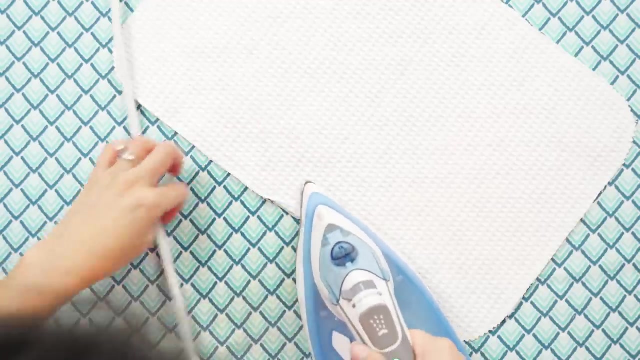 You may want to go slowly navigating those corners Back. stitch at the beginning and end With pinking shears. trim down the corner sections, Press back the seam allowance at the opening, Turn the cloth right side out and poke the corners with your fingers. 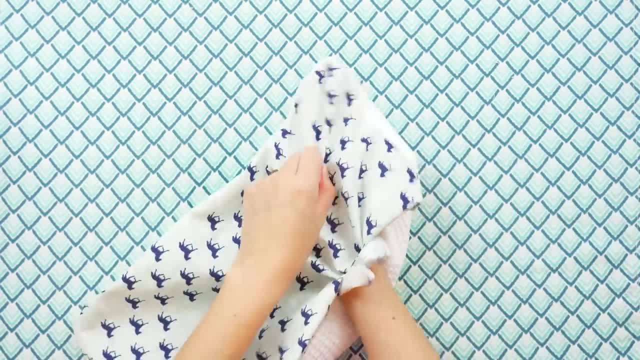 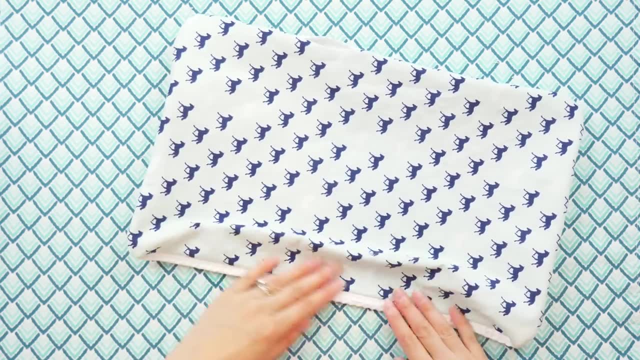 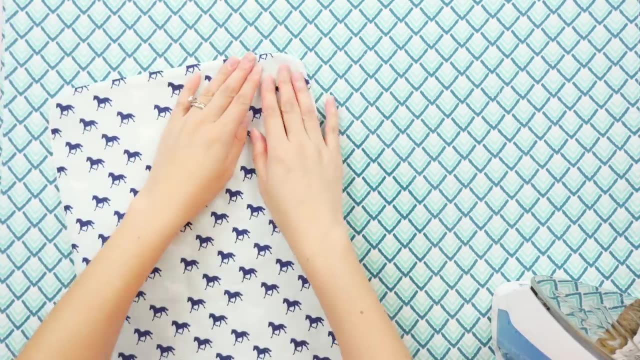 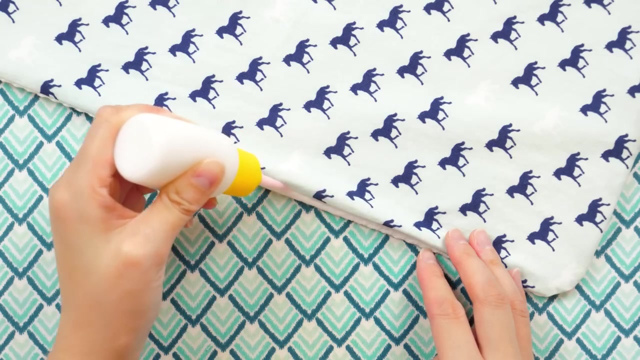 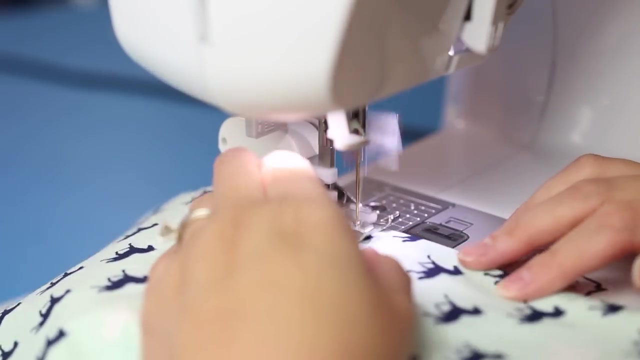 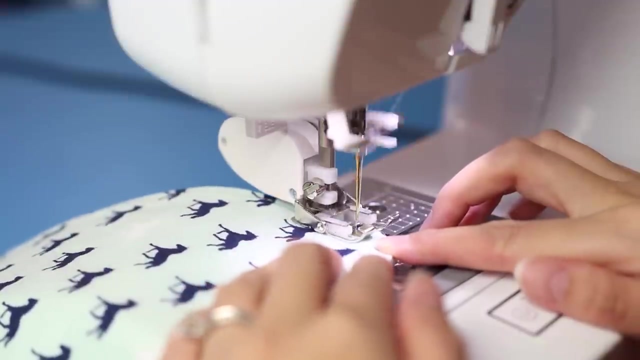 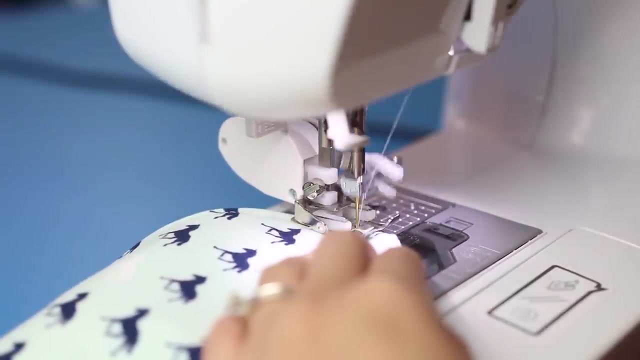 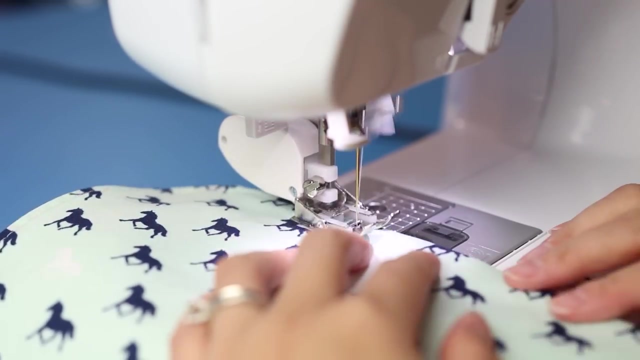 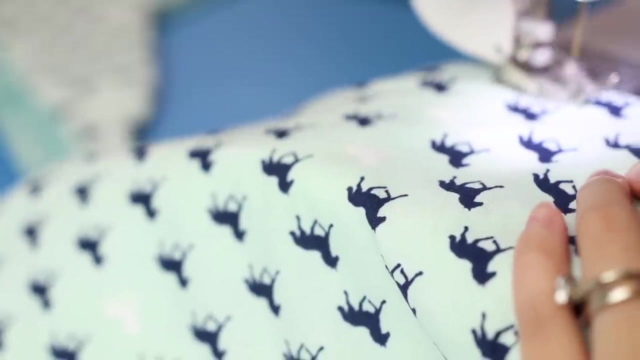 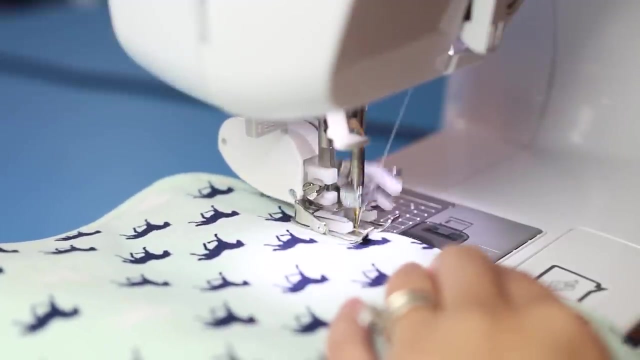 Push out the seams on each edge the best you can, then press, Use glue to close up the opening Top. stitch around the perimeter About a half inch away from the edge. Max the seam allowance. Turn the cloth right side out and poke the corners. 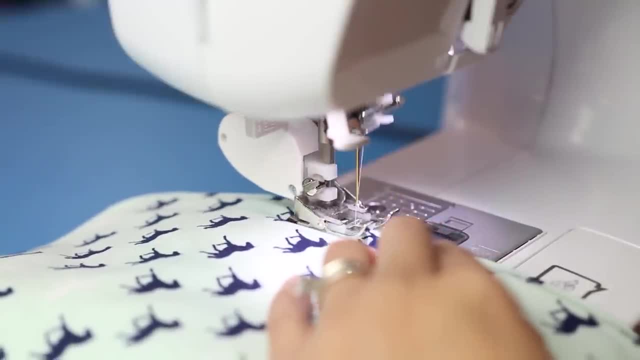 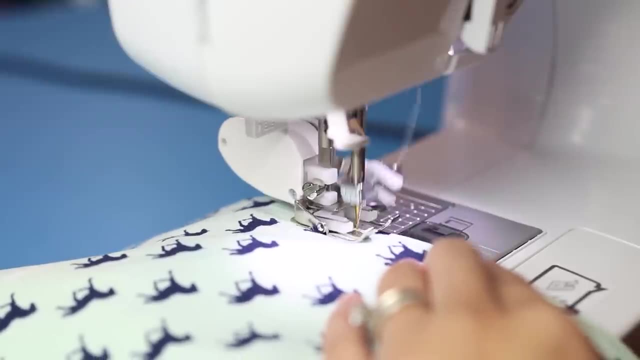 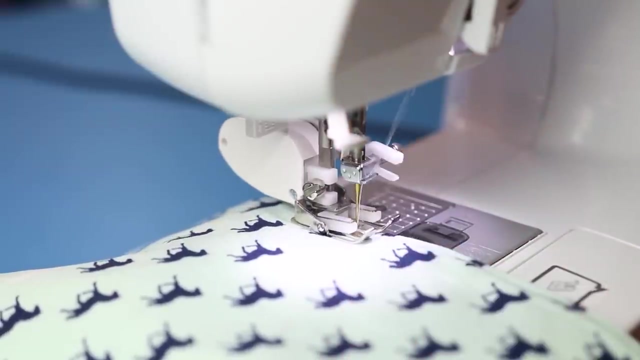 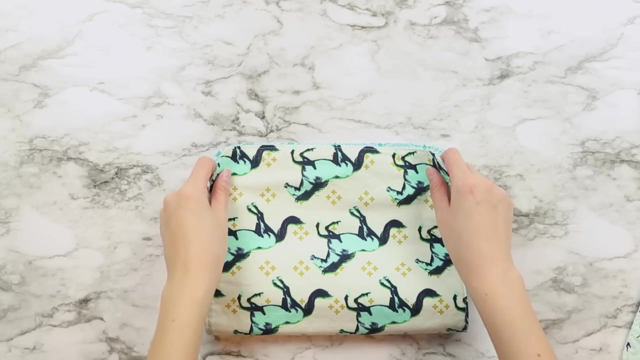 Use glue to cross out the money. Overlap the stitches a few inches when you get to the starting point to lock those stitches, Then fold down. These home cloths or unpapered towels are multi-use, anything from cleaning to baby burp. 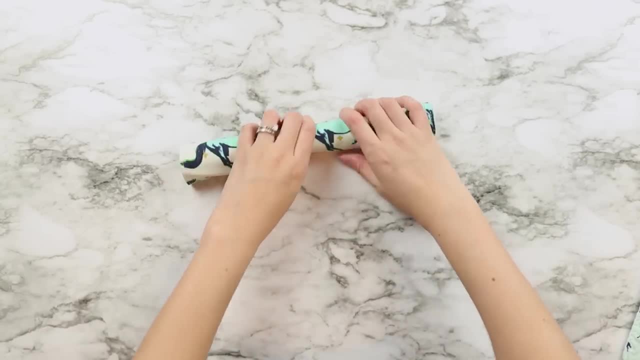 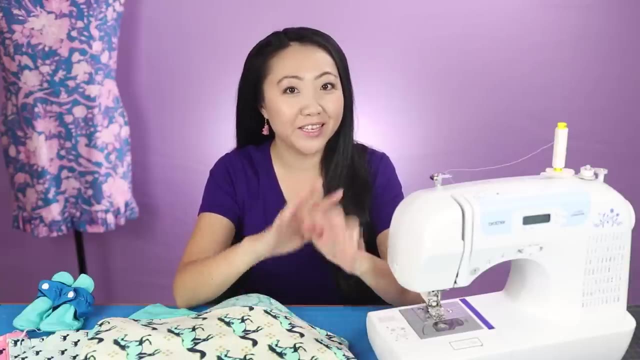 cloths. One idea for presentation is to fold it in half, roll up and display in a bunch. Oh yeah, and this project is fat quarter friendly, Okay. so, now that we've gotten through all of the gifts, I'm going to be wrapping them up, trying to maybe make them look somewhat presentable.